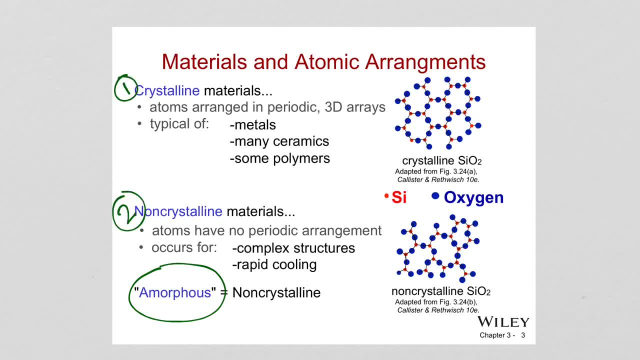 Okay So one, two, three, four, five, six, seven, eight, nine, ten. Okay So one, two, three, four, five, six, seven, eight, nine, ten, Two. So crystalline means there is the atoms in the crystal. they are arranged in a periodic way. 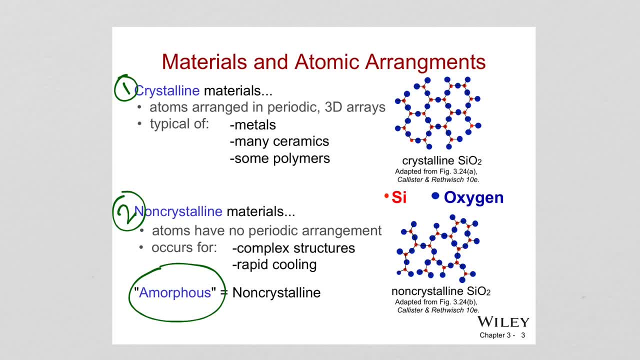 Okay, So the neighbors of an atom always the same throughout the structure. Usually metals, ceramics and polymers can be a crystalline structure. There is the crystalline silica. image is shown. As you can see, if you look at this atom and go somewhere else in this structure and find the same atoms, neighbors are going to be the same right. 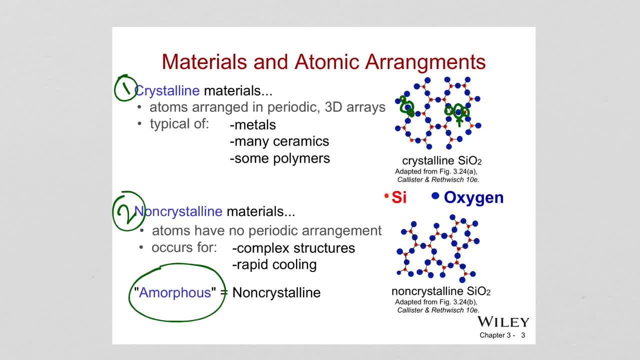 So wherever you go, look around you, there's an atom and you will see the same neighbors. So in 3D space you will always have the same atomic arrangement throughout the space. Okay, So these are crystalline. 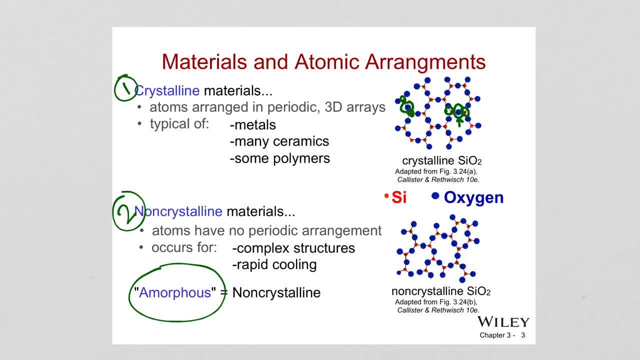 Non-crystalline. Non-crystalline: there is no periodic arrangements, So your neighbors can change when you go walk along the structure. okay, These are complex structures, usually achieved by different cooling rates. okay, If you don't let it give time to the atoms enough time, then they won't be able to go. 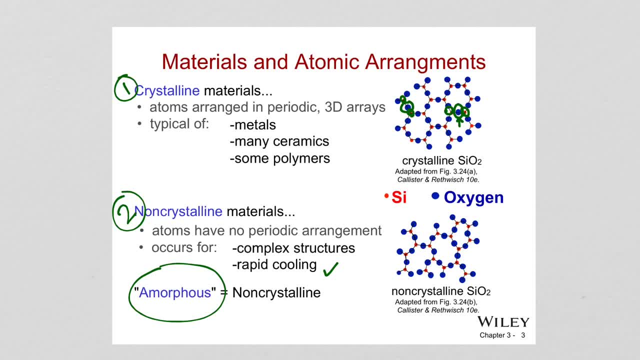 to their equilibrium places. Therefore usually rapid cooling, when you don't allow more time to those atoms to diffuse to their equilibrium places. Okay, That's where we observe non-crystalline materials And that is also called amorphous. 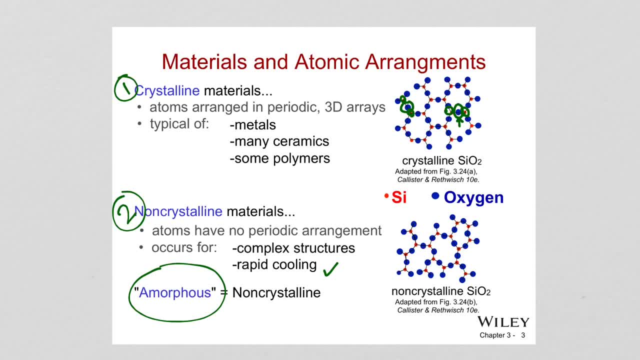 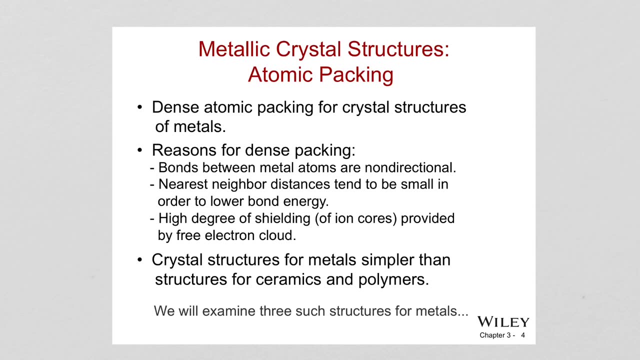 And, as you can see, the same silica structure can also have, in addition to crystalline, they can also have a non-crystalline arrangement. So when we look at metals, we see a dense atomic balance. Okay, Okay. 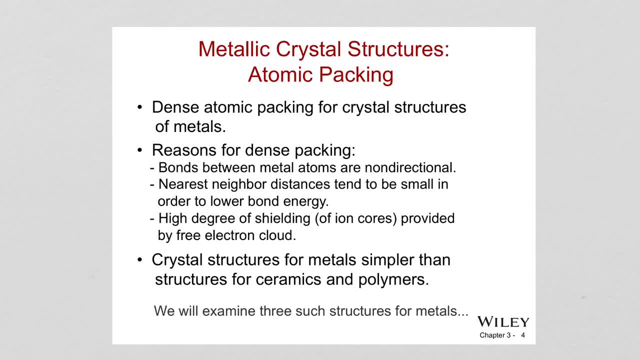 So the atoms can be in all directions, So, therefore, this means, therefore, they can have large amounts of potential. Okay, Okay, So these are non-crystalline. So, these are non-crystalline. 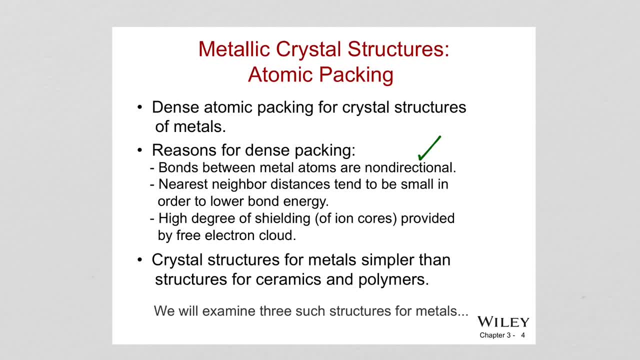 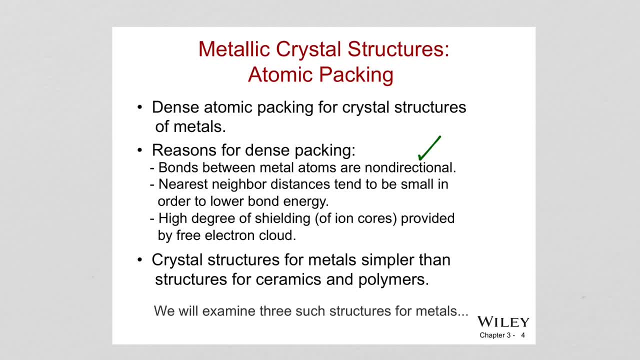 Okay, Okay, Okay, Okay Okay. numbers of nearest neighbor atoms, because the atoms can approach in all directions, right. therefore they are experiencing a dense packing. so dense packing also means basically low bond energy, or they are more stable, basically okay. and since there are three electrons in the structure, this shields the 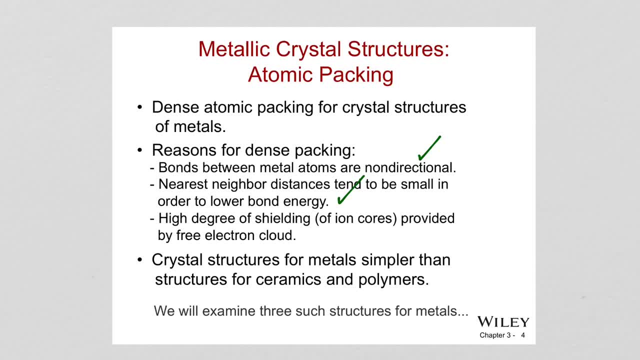 ion cores and they they are basically more together packed- okay, more densely packed together- crystal structures of metals. compared to ceramics and polymers, it is much simpler, easy to imagine and 3d easy to sketch and therefore we will look at three different structures for metals, how they can pack in space in 3d. 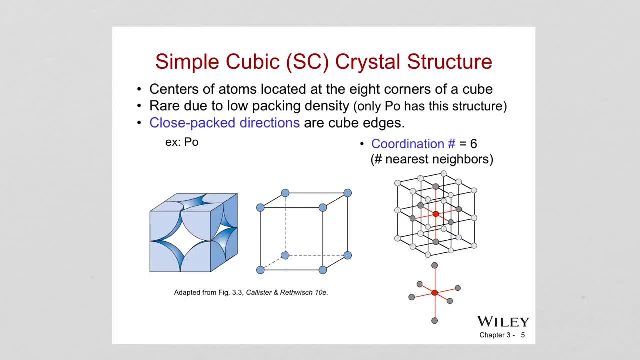 you. so this one, first one, is simple: cubic structure. okay, so when we are showing the crystal structure, we can use several different illustrations here. the first one is showing us a hard sphere, unit cell representation. so first of all, we need to understand what are units cells. basically, unit cells are described to describe the overall crystal structure. 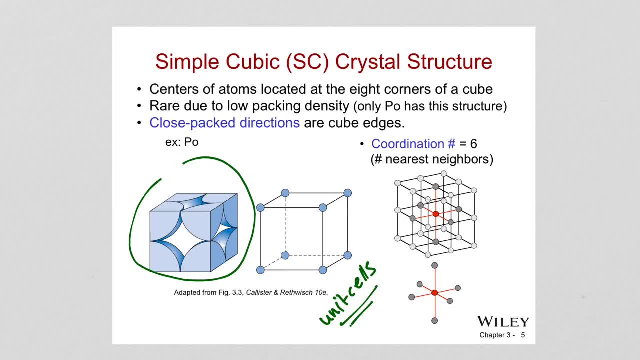 and how they part in 3d. this is the smallest repeating unit in the crystal structure, so you need to add up these structures in space together to imagine the overall atomic crystal structure. so we are slide to do double through from what we have shown on the shaded screen part of this picture. what allow us to chose 2d channel? of theиту numeric configuration. so this says 3d in each years, one unit cell, so a single n is becoming the focus of the entire load unit storage. Brazil is will copy this and this is what we have shown in the complete material, but they may still mesmo hip is repeated in mı, so there are multiple ways you could incorporate these�. 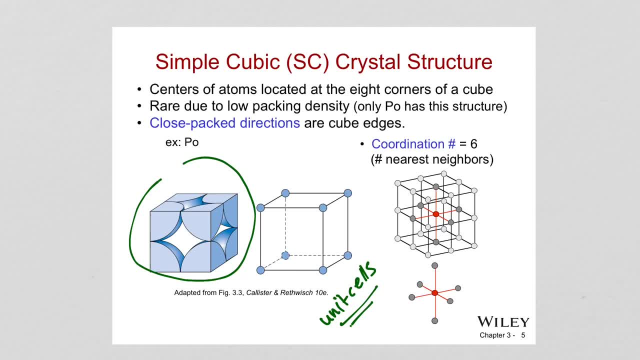 okay, so this is basically the smallest repeating unit, the unit cell, and there are ways to show it. this first one is called the heart sphere unit cell representation, and this is reduced sphere unit cell representation. as you can see here, in reality the atoms are touching each other, but we can also 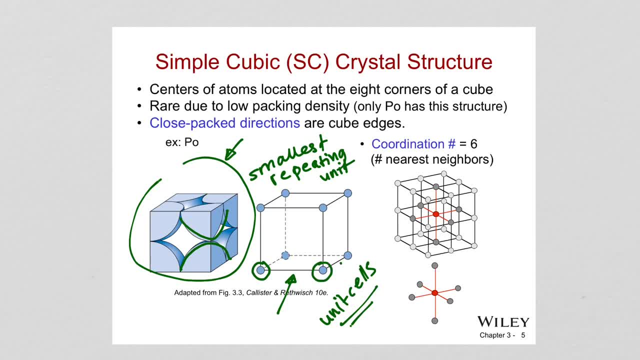 represent them this way, putting them at the corners of the unit cell. so in simple cubic the atoms are located, the center of the atoms are located at eight corners of a cube. okay, so we that means we have eight atoms at each corner of a unit cell. this configuration is rare because it doesn't give low packing density meaning. 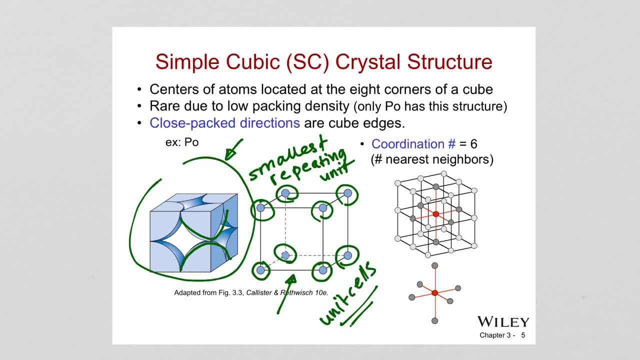 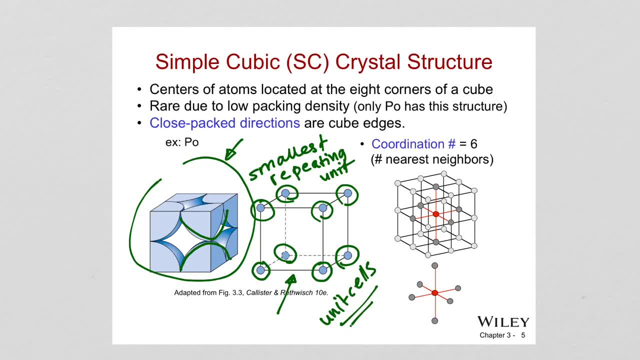 the coordination number six is giving us the nearest neighbors. so if we look at an atom in our unit cell, nearest neighbors will be one, two, three, four, five, six. okay so here so these. even if it's shown like these atoms are separate to each other, in actuality they are touching each other like that. okay so? 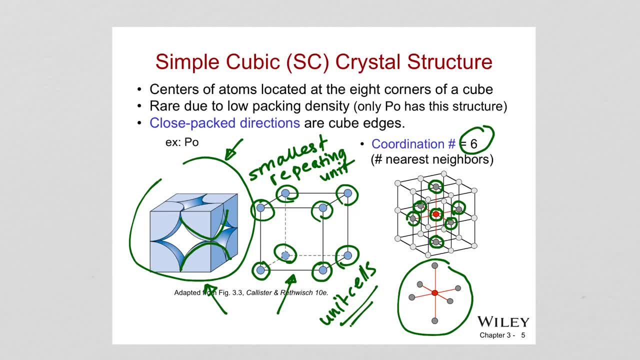 those are the nearest neighbors of any atom in that repeating unit. so we have eight atoms, but within the unit cell only one over eight times of an atom is within the unit cell, right this corner here. this part is one over eight times of a single atom or a single point in the unit cell. therefore, 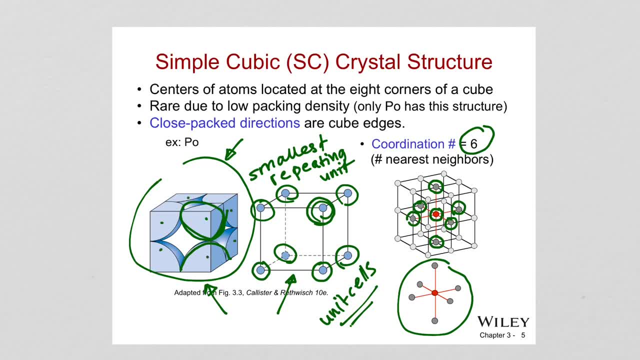 overall, if you sum all these up together, they will make just one atom. so actually there is only one atom within a unit cell, so eight at the corners, but only one over eight times of those individual atoms. So we have eight atoms. The individual atoms are in the unit cell, so this gives us one. so total of one is in. 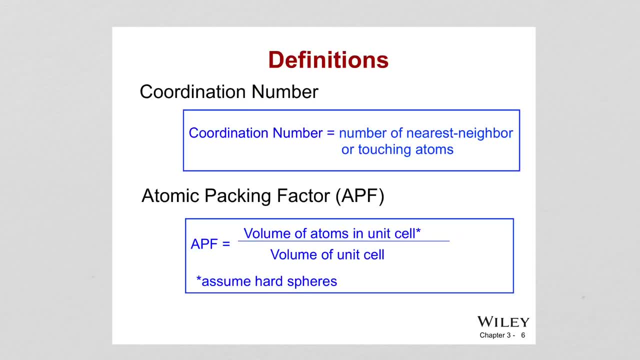 the unit cell. So how the coordination number is found, as we said, it was six in the simple cubic structure it is the number of nearest neighbor atoms that are touching- okay, touching to each other. and there is also atomic packing factor Which gives us information how well packed atoms within the unit cell and, of course, throughout. 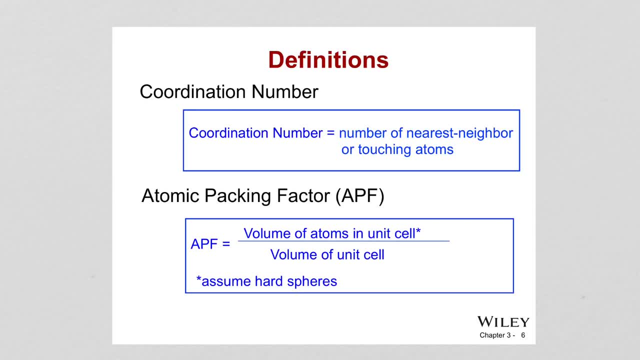 the structure therefore- So this is defined as: first, find the volume of atoms in the unit cell- okay, what is the volume of atoms in the unit cell- and divide this to the volume of the unit cell and this will tell you within the unit cell and therefore in overall structure. 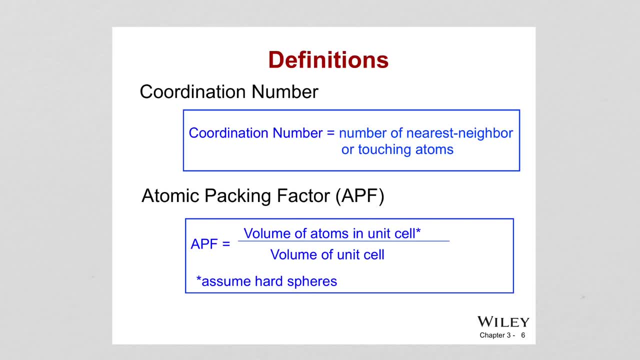 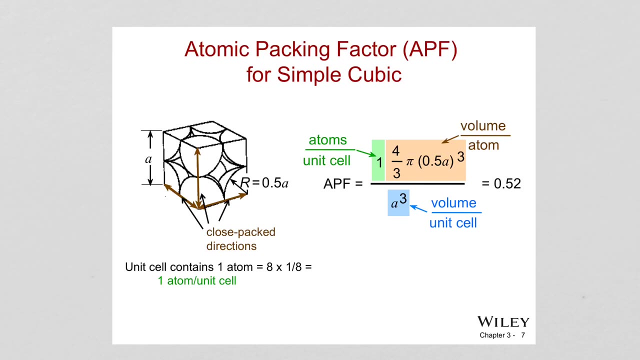 Okay, What is the atomic packing factor? and of course this is going to be different for different structures, different unit cells. So in this case, for the simple cubic, if we look at how we can calculate the atomic packing factor, first you guys need to figure out how many atoms are there in a simple cubic. 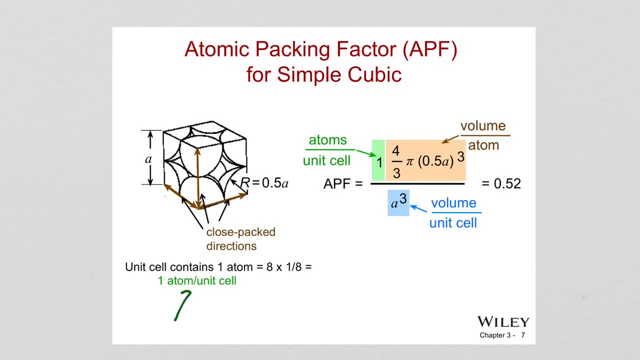 Structure. so, as I explained to you guys, only one over eight times of an atom is inside the unit cell and this is that corner. each corner only goes normally. normally, the atom is like this right, And only one over eight of this is inside the unit cell. 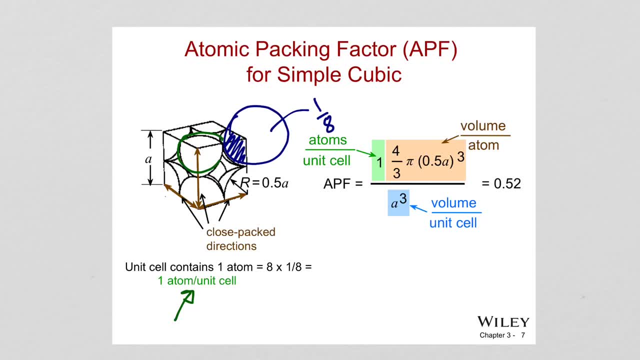 Okay, Okay, Okay. So therefore, even if you have eight atoms at the corners, only one over eight of it is in. Therefore, since we have eight atoms, then we need to multiply eight times one over eight. so there is one atom per unit cell. 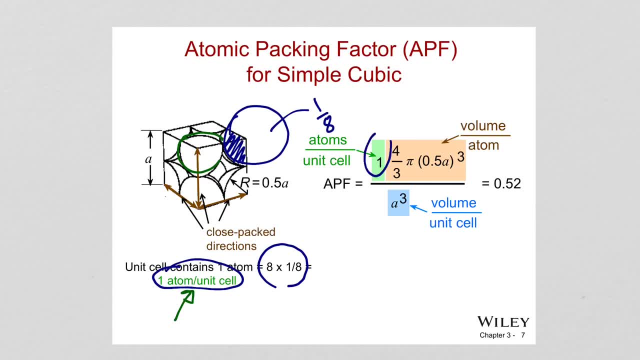 Okay, So first we found one atom per unit cell, And then we need to find the volume of atoms in the unit cell. Okay, And then we need to find what is the volume of this? Of course, volume of an atom is- you can think it as a sphere- right? 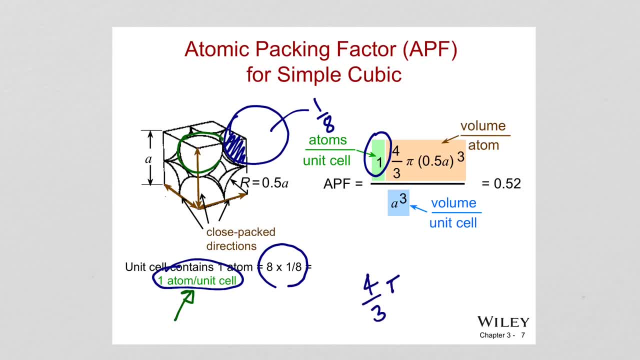 So sphere volume is four over three times pi, times r to the third. So, therefore, what is the r, what is the radius? and it will be given to you in terms of atomic lattice dimensions of the unit cell. Okay, So a is basically a unit cell dimension, right? 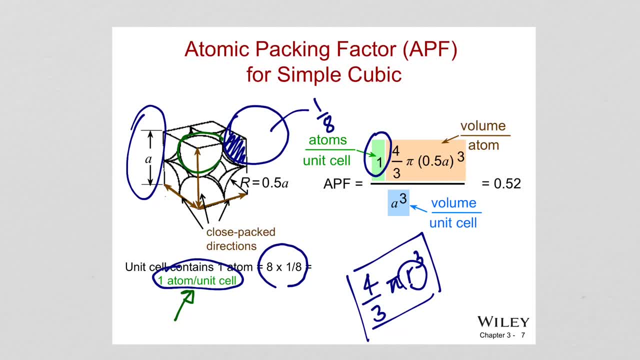 One side of this unit cell And r is going to be, of course, the half of it, Because, since these are packed together closely, as you can see, these two packed together right, There is no empty space in between them. So the overall edge, this one will be equal to two r. 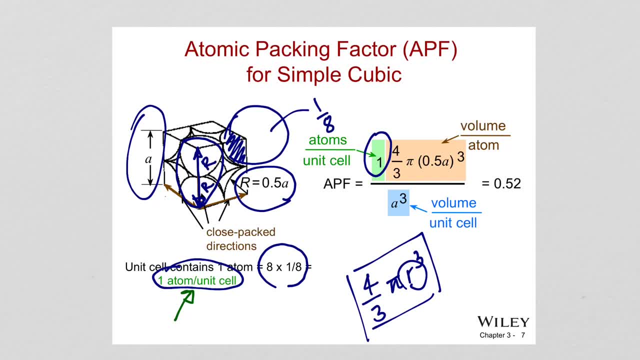 Okay, Okay, So r is equal to two r's, or therefore a is two r, or a r is one over two a. Okay, So therefore, if we want to represent r in terms of unit cell dimensions, here we can plug in point five a, like we did here. 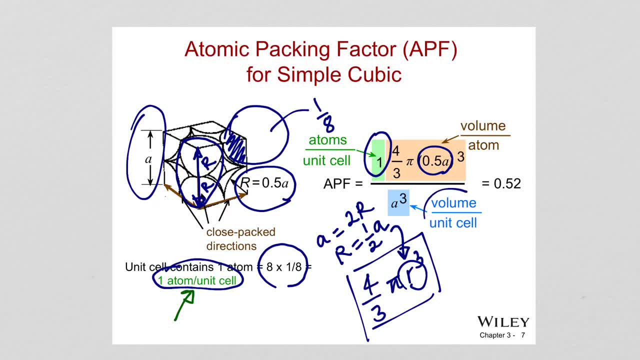 So what is the volume of the unit cell? The unit cell itself is a cubed because it's a cube, right? A cubed is the volume of a cube And what is the packing? therefore, Since a is going to cancel each other, you can find it's going to be point five, two, for 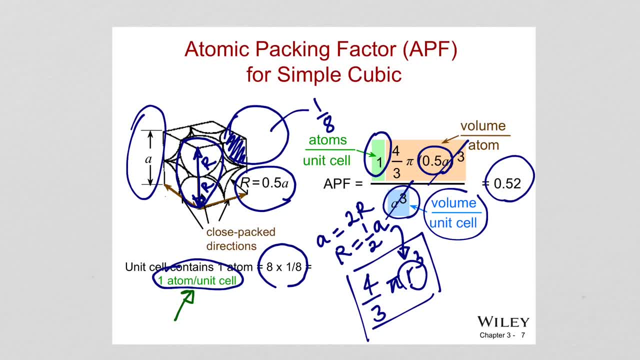 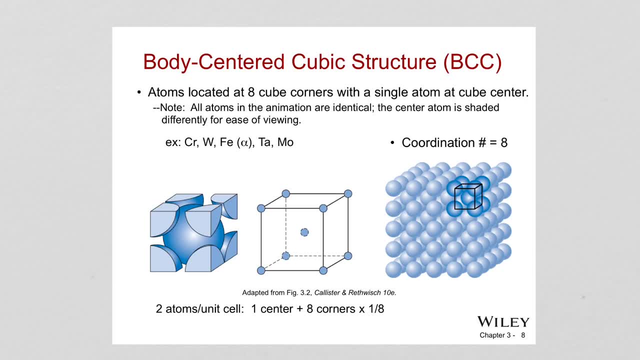 a simple cubic. Okay Now another crystal structure Is body centered cubic structure. In this case, beside having atoms at the corner of the unit cell, we also have a center atom like this one, And of course you can see unit cell here is representing the smallest unit, that is representing 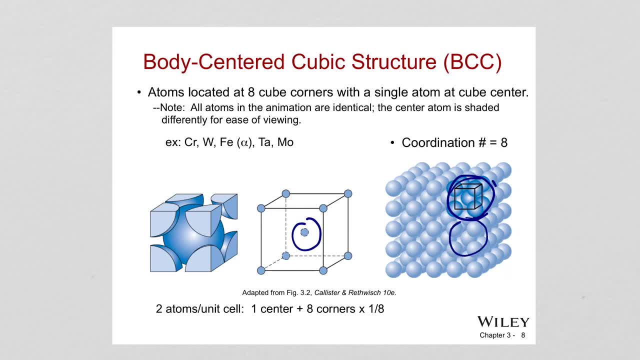 the overall crystal structure, and this thing repeats over the crystal structure again and again. So we are building the 3D structure of the overall material, But working with the smallest unit, we can understand the overall structure And therefore that's what we are doing here. 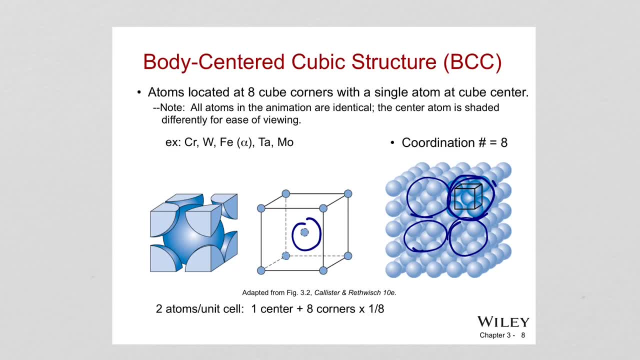 And this is the BCC, which has the cube, which has the atoms at the corners and a single atom at the center: One, two, three, four, five, six, seven, eight at the corners. And one, two, three, four, five, six, seven, eight at the corners And one at the center. 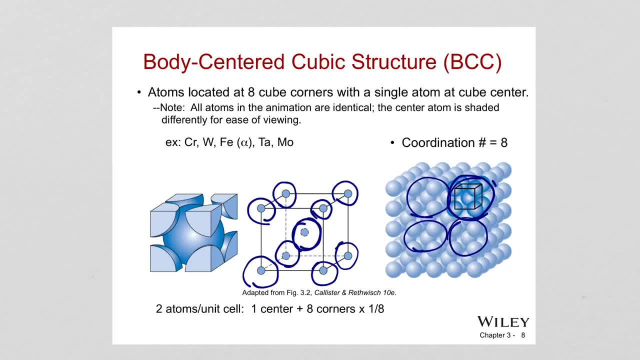 But how much of these atoms are actually within the unit cell? As we see again, only one, over eight times of each atom is within the unit cell, And all the whole atom is at the center. Therefore, therefore, in this case, How can we calculate? 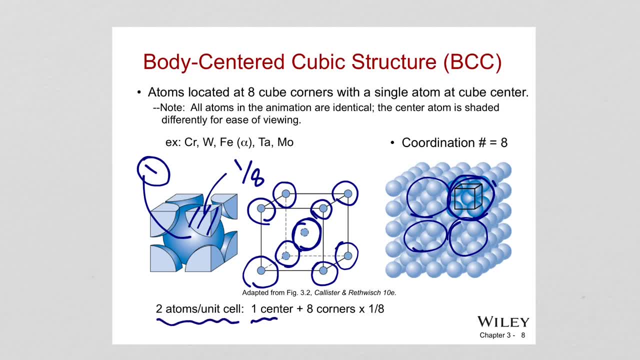 Here it is number of atoms in the unit cell. one is at the center, eight times one over eight is inside the unit cell. so one or plus one, which makes actually only two atoms per unit cell. so coordination number is what in bcc, if you guys think about it? uh, how to add how much? 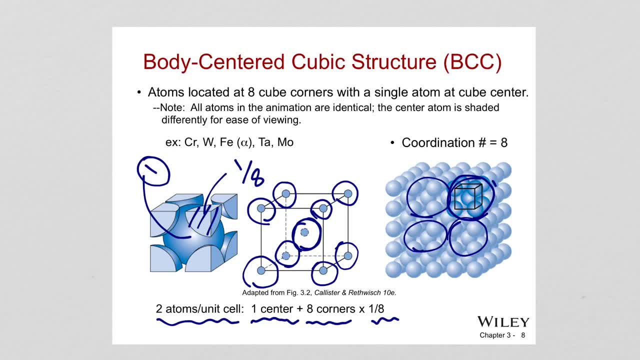 atom is touching the center atom. you can see that one, two, three, four, five, six, seven, eight. so the coordination number is actually eight nearest neighbors. okay, so what type of structures, what type of metals have this? uh, this is not a very mostly packed structure and we can see if we calculate atomic packing factor compared to others. the reason is usually: 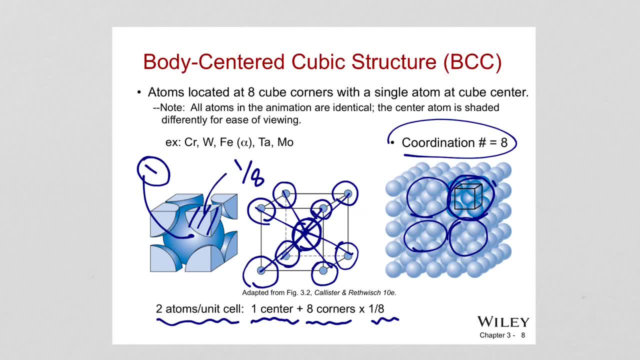 these metals experience covalent bonding, which is a directional bonding besides metallic bonding. therefore, the packing is less as compared to other highly packed structures, and the materials that experience this type of packing is chromium, tungsten, iron, but some type of iron, alpha iron and et cetera. so, uh, the main reason tungsten has a high melting point is therefore, as i explained. 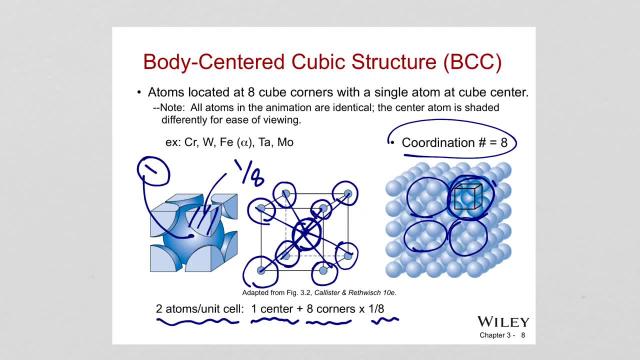 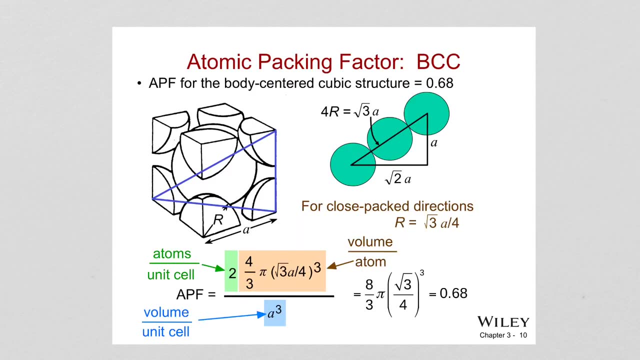 is having a problem bonding in the structure as we talked about it, and therefore it is experiencing bcc structure. so if we try to calculate here the atomic packing factor, factor for BCC structure, let's do it. so we know there are two atoms in the unit cell and what is? 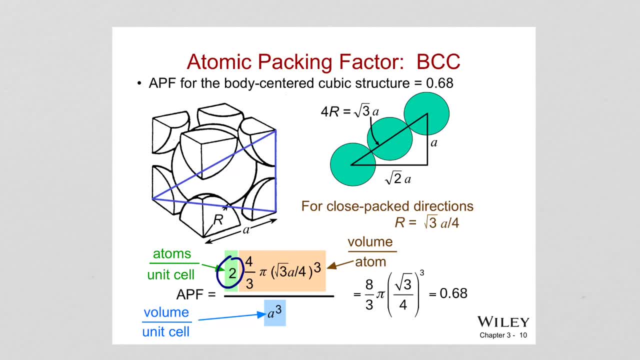 the volume of each of these atoms. so you need to find a correlation between R and a. so a, we know the lattice dimension here- unit cell dimension. a- what about our R is the radius of the one Adam. but to make this correlation you need to find the densely packed direction. 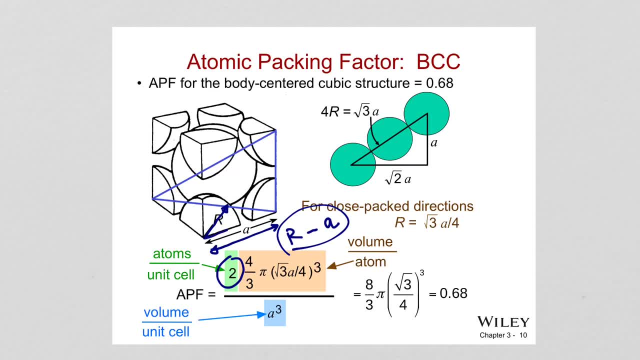 okay, and that's the packed direction is not here, as you can see, because there is an empty region here and we cannot make a correlation between R and a, the, the, the. the line that we can make a correlation between R and a is the diagonal, because the atoms are. 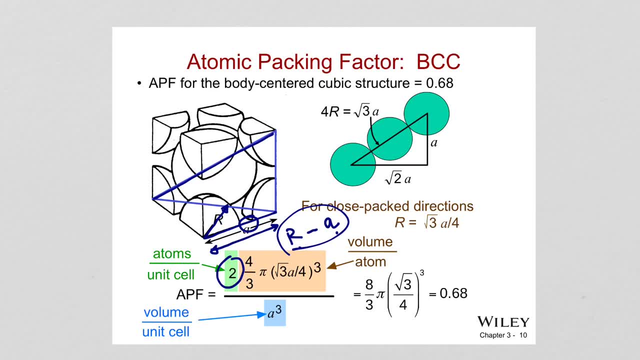 packed with no empty space. how they are packed along the diagonal. if you look at, this is a here. okay, and this one is square root of square root of 2 times a. how come? because this is a, this is a. this is square root of 2a. 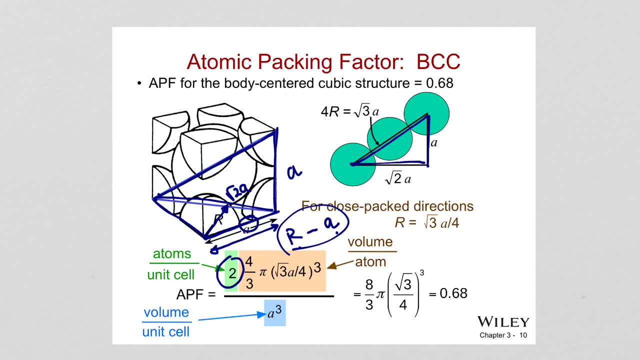 so, therefore, we are seeing the triangle here right, and this is the diagonal. so what is the diagonal it has to have? it is R of 2, 2R, so overall 4 R. And what is this one? Of course, you can find it from hypotenuse theorem. You can find it right. So what we do? a squared over. 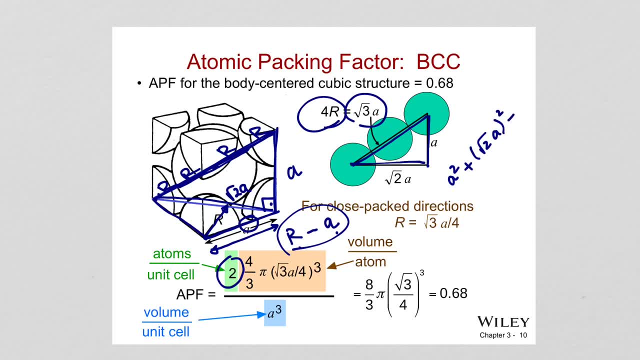 So what is that? x, right, Okay. so that means 4r in the diagonal is equal to square root of 3 times a, and there is this relation, therefore, between r and a Instead of r. you can write this down and figure out what the volume of an atom is. 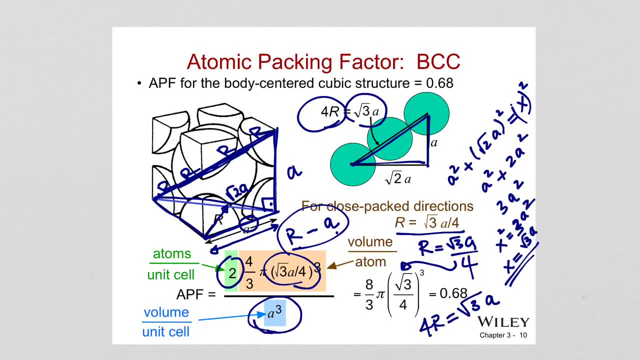 And we know the unit cell volume. It is a cube's volume, a cube, And therefore you can calculate atomic packing to be 0.68, which is, as you can see, better than 0.52.. So better packing in the BCC compared to simple cubic structure. 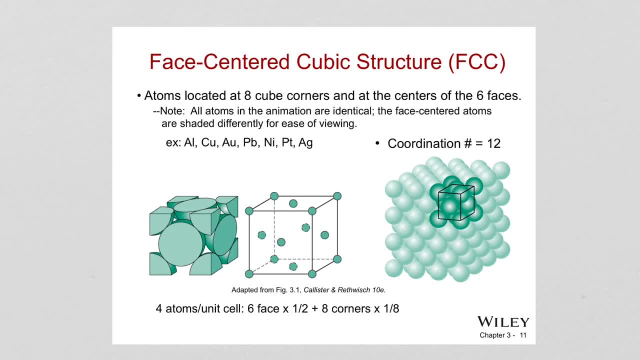 So FCC is what we call face-centered cubic structure And it is a highly packed structure, In this case usually atoms, usually the metals that are experiencing FCC type of crystal structure. These are aluminum, copper, nickel, gold, silver. Okay, so this type of packing in the unit cell atomic model is short. 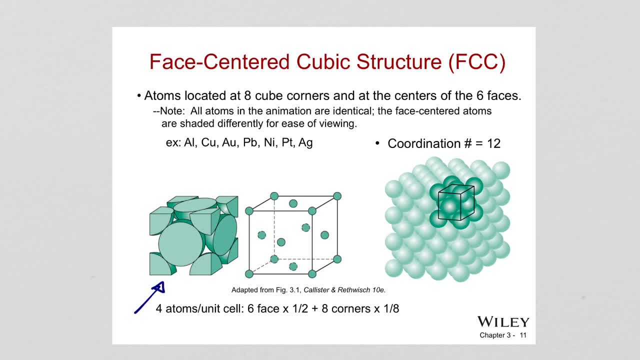 The difference here. at each face of the cube, the unit cell, we have an atom And of course the cube will have six faces right. So therefore, only half of the atoms in each face will be inside the unit cell, as you can see. 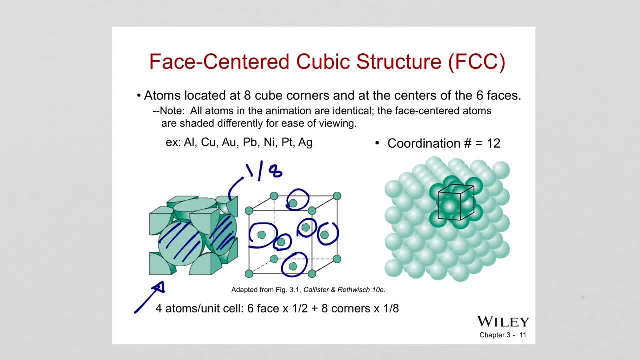 So for each corner. So for each corner only one over eight times of each atom, and for each face one over two times of each atom. So since we have six face and one over two, just three of the atoms are in the unit cell. 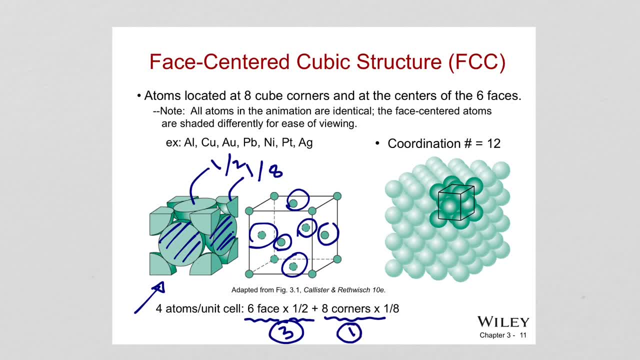 And eight times one over eight. one of them is in the unit cell, So in total there is four atoms per unit cell. So to understand the coordination number for FCC you guys need to do some imagination in 3D okay. 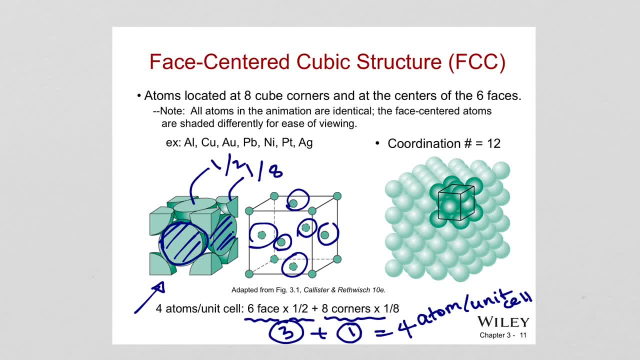 So I'll try to explain. So think about this one in 3D full atom. It is touching one, two, three, four, On the back five, six, seven, eight And of course on the other side it's going to be four more right? 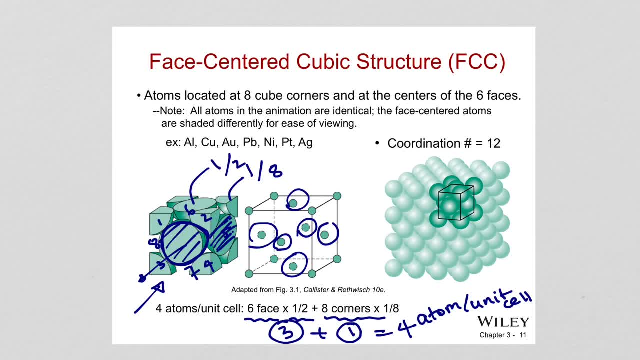 Four more eight plus, because there's going to be these again on the other side. So there's going to be four more eight plus four, twelve. Okay, So twelve. the coordination number is So if you have guys having hard time imagining this, I would just Google the coordination number for FCC. 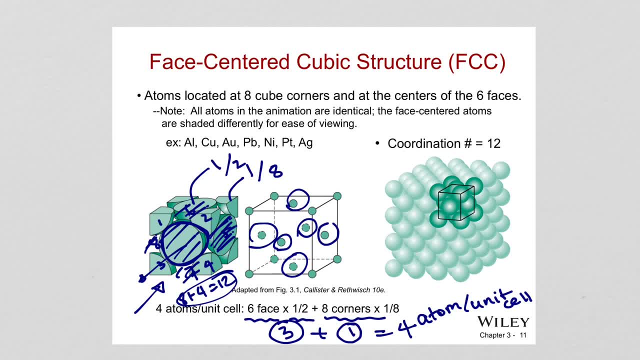 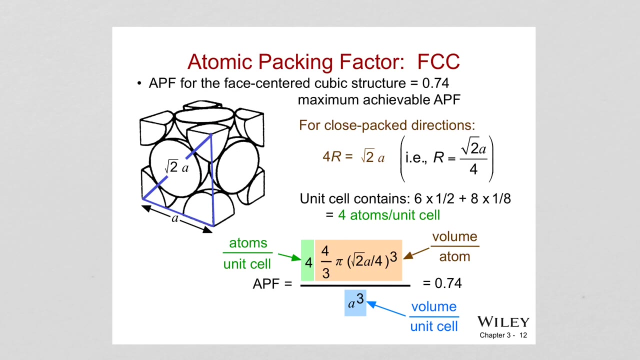 and look at the images, because people provided images for better visualization. Okay, So the twelve is the coordination number And four atoms are there in the unit cell. So when we look at FCC- atomic packing factor- again, what we need to do is put: 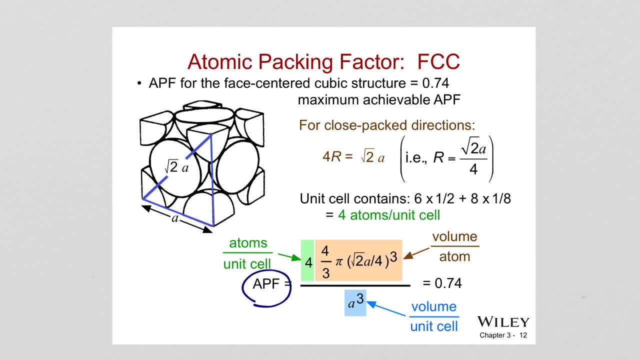 to calculate this atomic packing factor, we need to find the terms in our equation And we now know that there are four atoms. Okay, There are four atoms in a unit cell And the volume of each atom is a sphere volume, basically. 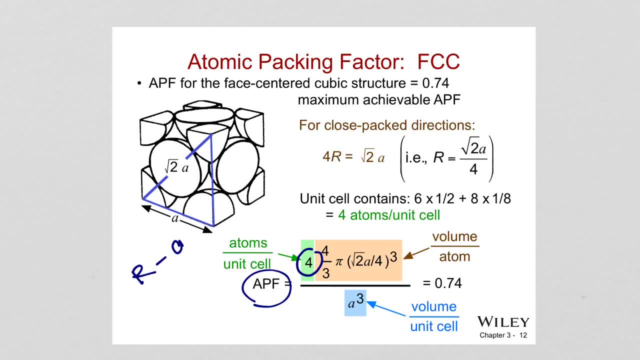 But to do that, we need to find the correlation between R and A And, of course, we need to find the most packedly, most densely packed direction, And it is in the diagonal of each phase, which is, of course, this is AA and this is square root of 2A. 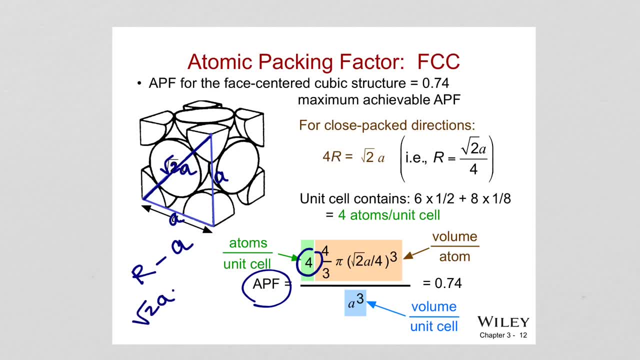 Right, Okay, So the square root Of 2A is also equal to R, 2R, R, So it is 4R. So that means is basically: R is square root of 2A over 4.. 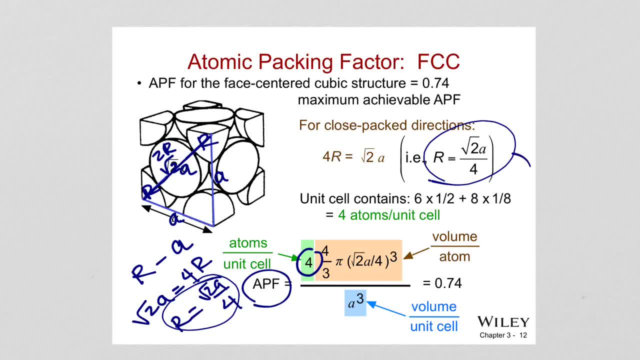 This is what is given here, And then we need to plug this information in our sphere volume equation- Okay, And after we do that, so we need to figure out how much these atoms are. Okay, So we need to figure out how much this atom space is occupied within a unit cell. 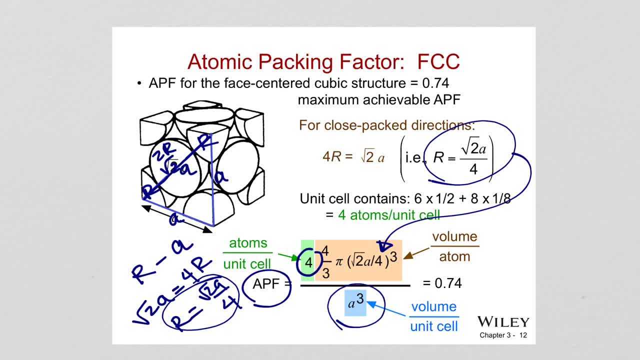 So we need to know the volume of the unit cell And the result will give us 0.74 as the atomic packing factor, which is higher than 4.. It is 4 simple cubic, and it is 4 BCC. Okay, 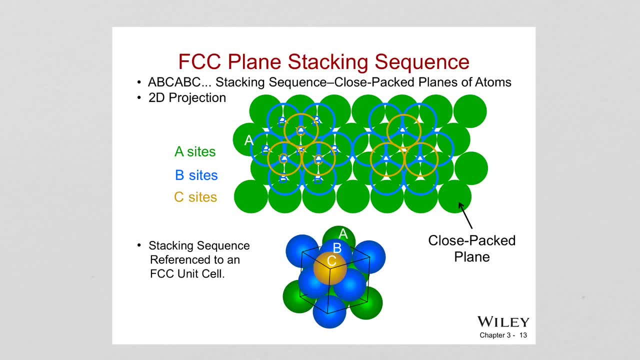 So we need, in order to understand how the atoms can pack Very densely in FCC, we need to do some imagination in 3D, Okay, So we're going to start with putting atoms together as densely as possible. Think about you are placing ping pong balls together. 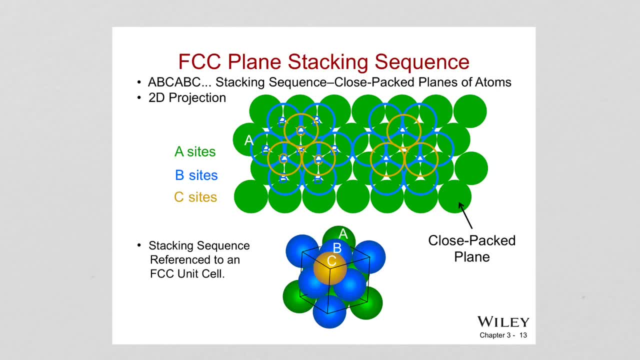 Okay. So what we could do in order to pack them very densely right, So we could fill up every empty space. So this is like, say, first layer we are putting is A Okay, So I would put here and then put here and then fit in one here. 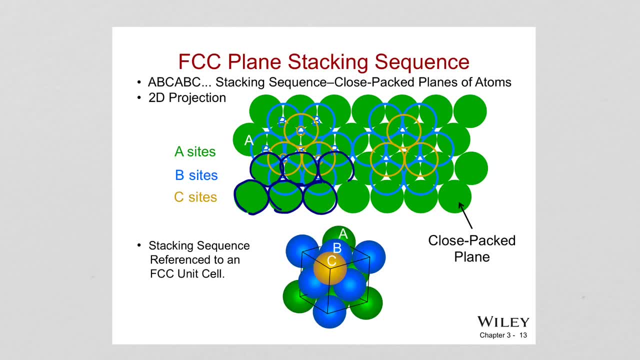 So they are touching everywhere each other. right? This is A. So what I do, I would do further in space. I would now find the empty regions where I can fill with extra layer of atoms. So on top of this, now I can put atoms B to empty spaces. 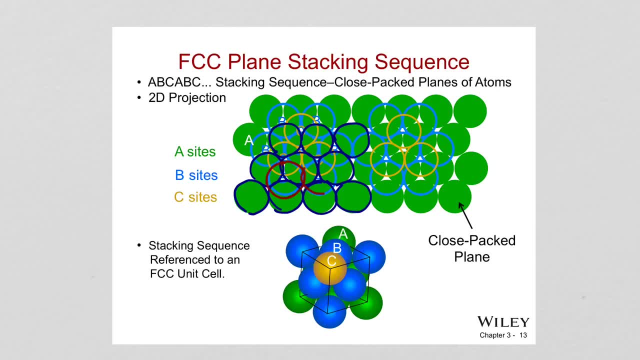 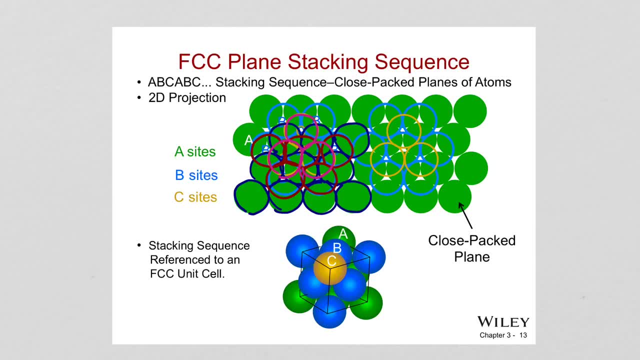 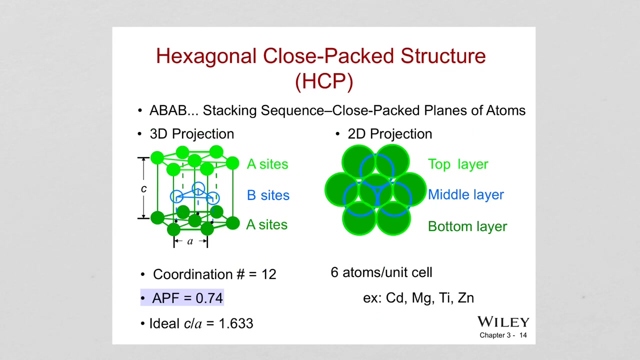 Et cetera. So this is just showing you How well atoms packed in an FCC structure and it just requires some 3-D visualization. That's it So: hexagonal closed packed structure. and this is another closed packed structure and this time the 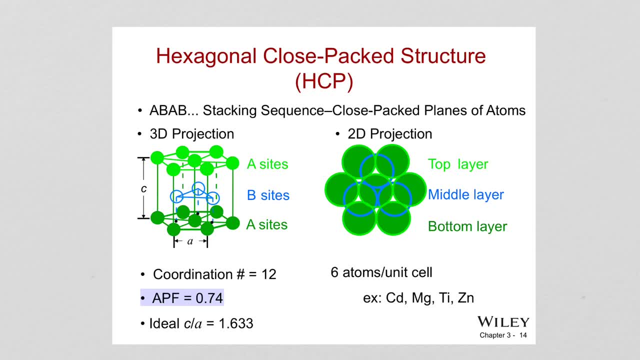 top and the bottom faces of the unity cell consist of six atoms that form a regular hexagon: One, two, three, four, five, six, And then they surround a single atom in the center, One. Okay, So one, two, three, four, five, six and one at the center. 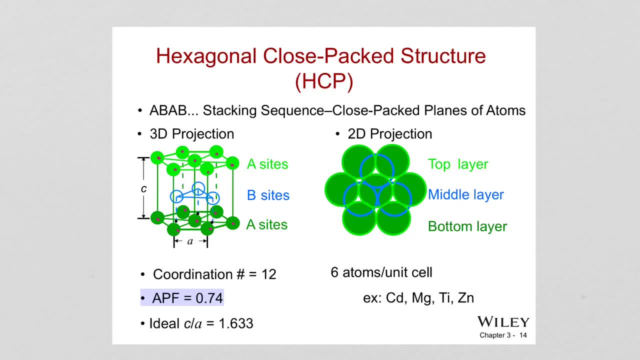 And there is another plane that provides three additional atoms At To the cell, which is in between the top and bottom planes. If you look at the number of nearest neighbor atoms, it's going to be 12 again, like it was in FCC. 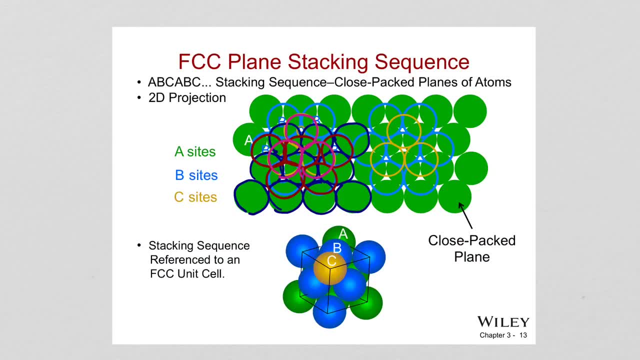 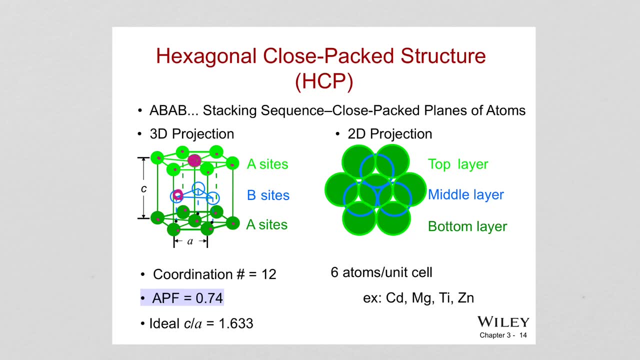 Okay, It's here, right, So you need to imagine. So think about this atom here which is touching to one two, three at the bottom. One two, three, Uh, at the top, and one two, three, four, five, six here. 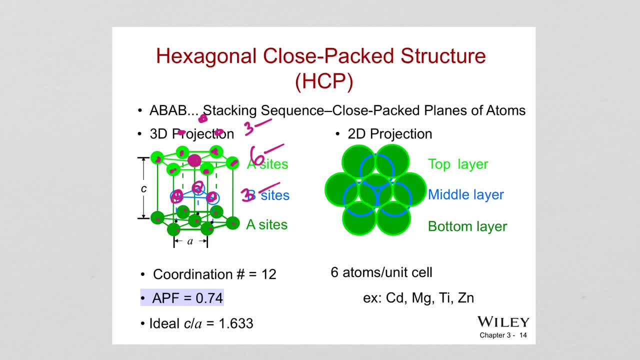 So it makes three plus six, nine plus two, three, 12.. Okay, And if you calculate atomic packing factor, it's going to be again with the same as FCC And there is an ideal ratio between C and A. Uh, that is found for HCP structures. 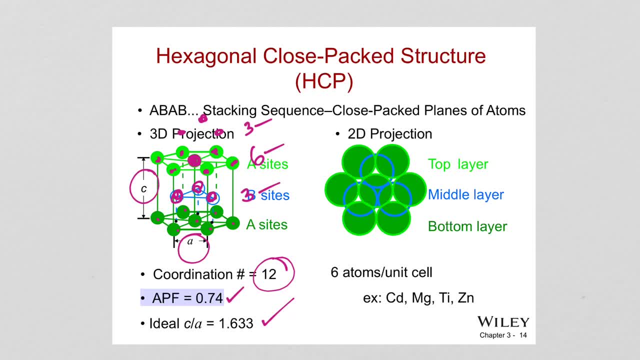 That is 1.633.. And there are six atoms in the unit cell, And there are six atoms in the unit cell. And there are six atoms in the unit cell, Why? Because three in the middle right And there are there are, uh, one and two active faces, but only half of it is inside. 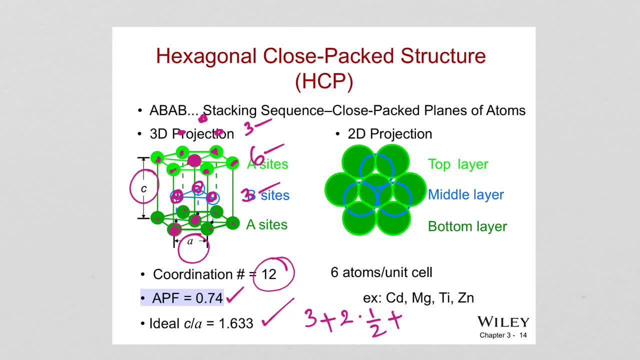 And there are 12 corner atoms: One, two, three, four, five, six, six, And then, on the top, also six, 12,, 12 times, only one over six, Because it's uh, Because it's uh. 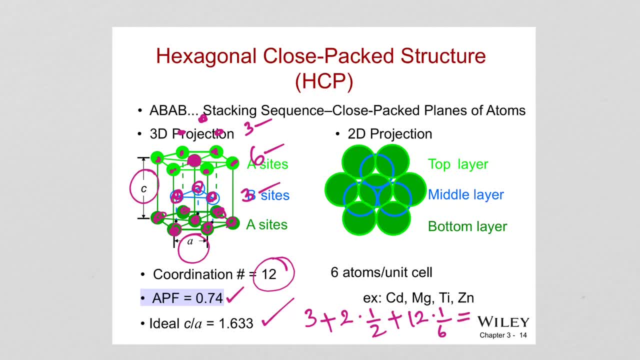 Because it's uh. The hexagon right One over six of it is in the uh unit cell. The hexagon right One over six of it is in the uh unit cell. That gives you six. 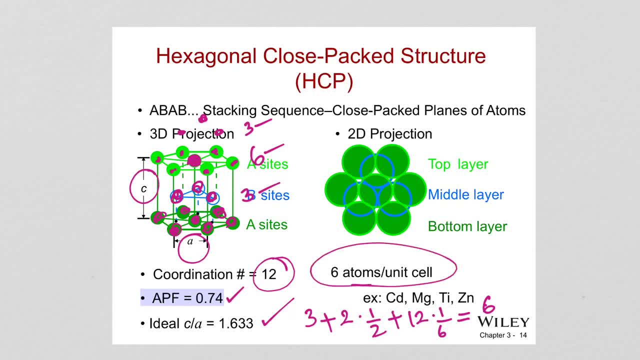 Okay, So, as you can see, the coordination number and then the packing factor is the same as the HCP, And certain FCC and HCP the same And certain FCC and HCP the same. So certain metals show HCP crystal structure. 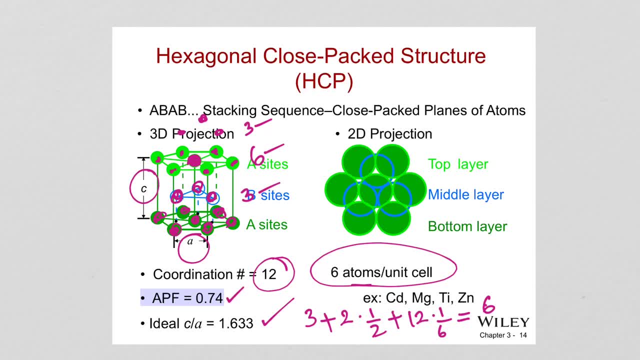 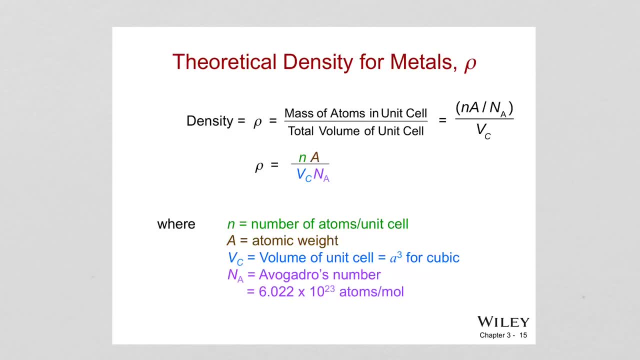 So certain metals show HCP crystal structure And certain File 몇 And certain File 몇 And certain File 몇. It's cadmium, magnesium, titanium and zinc. So how do we find density? So remember, density is not going to change with the size of the material. 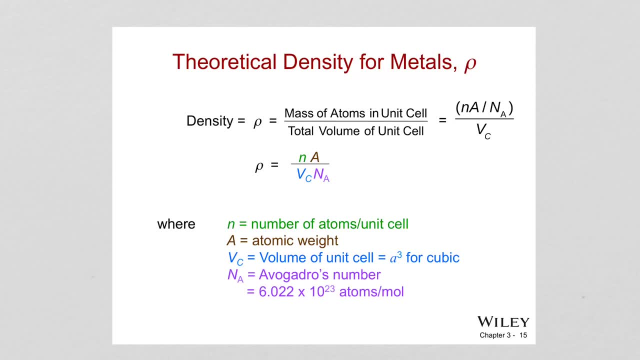 because it's always mass over volume. And if you actually can able to calculate the density of the unit cell, you can relate it to the overall density of the material. So, based on the unit cell, how we can calculate the density? So, first of all, there will be certain number of atoms per unit cell, right? 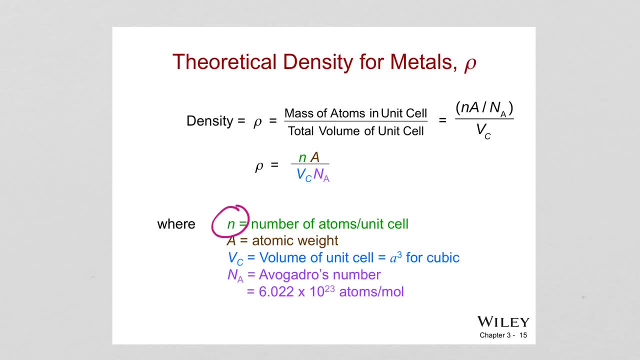 And what is the mass of these atoms in the unit cell, With the knowledge that we know, Avogadro's number of atoms has a certain atomic mass, Atomic weight, right? So this much of atoms or molecules, in this case, let's talk about atoms, right. 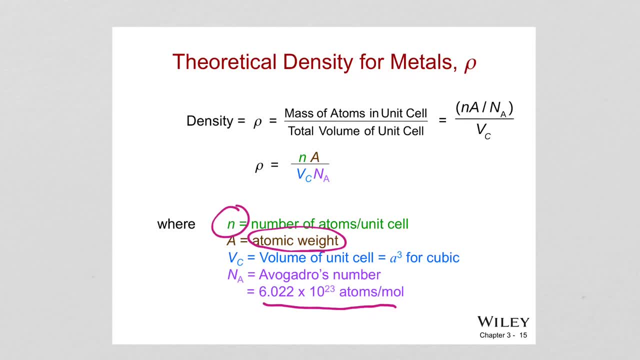 This much of atoms. let's say, if it was carbon it's going to be 12 gram per mole, right? So if we divide atomic weight to that, we can understand a single mass of a single atom. So therefore, if I need to multiply it with this, 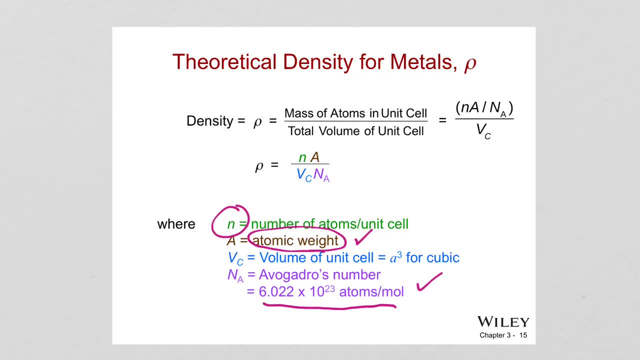 therefore, with the, with the how many number of atoms I have, So n times a over Avogadro's number, And on the denominator. of course this is mass and over volume. right, The density definition is that, so total volume of the unit cell. therefore it's easy to find. 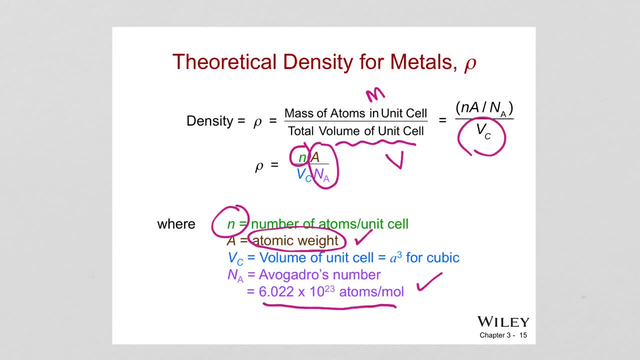 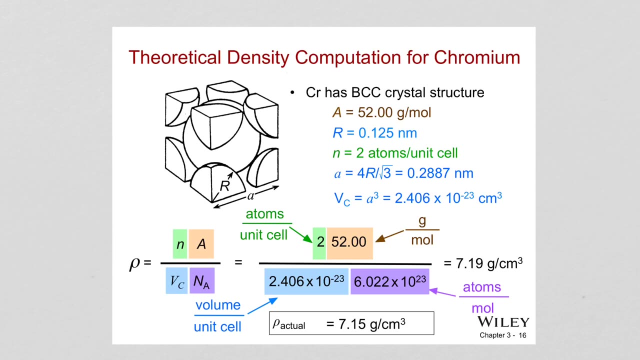 because we know it's a cube. Okay, From there we can figure out the density, theoretical density. So we are given an example for chromium. How can we calculate the theoretical density? First, you need to know the crystal structure, and chromium has BCC crystal structure. 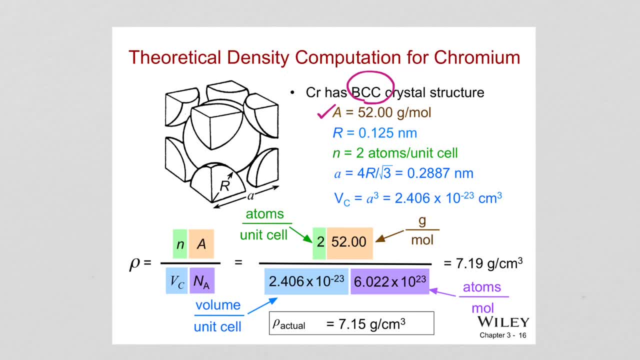 Atomic weight is 52 gram per mole. its radius is given 0.125 nanometer here for each atom. And then how many atoms in one unit cell? Of course you need to know this one If it's a BCC. you know there are two atoms per unit cell, and we also know the relation between A and R and 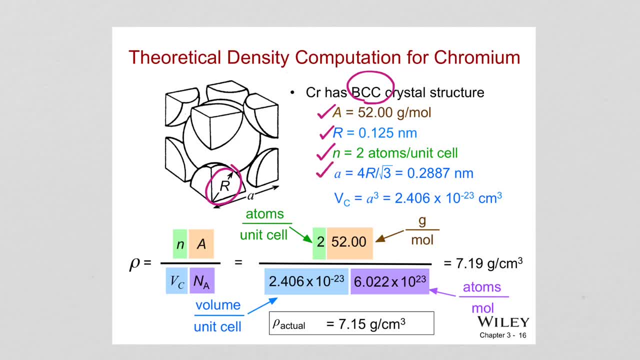 from that you can calculate a also. this dimension, unit, cell, cell dimension, since you know the r and the volume, is simple. right, it's a cube, so a cube. since you know the a, you just plug it in here and calculate the volume. okay, now all we have to do is: 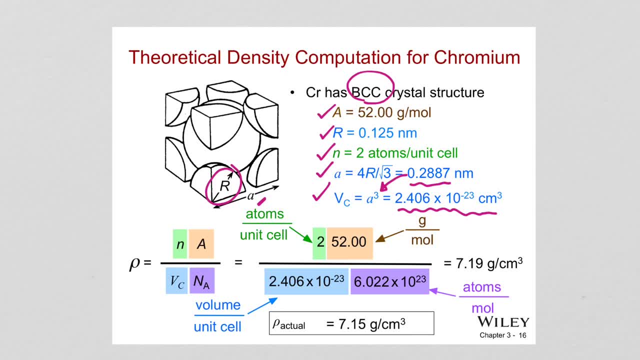 plug it in into the equation. so the density here, which is we need to multiply it with number of atoms, which was two times the atomic weight and times the over the Avogadro's number and over the overall volume of the unit cell, and this gives us seven point one nine. so actuality, this can be very. 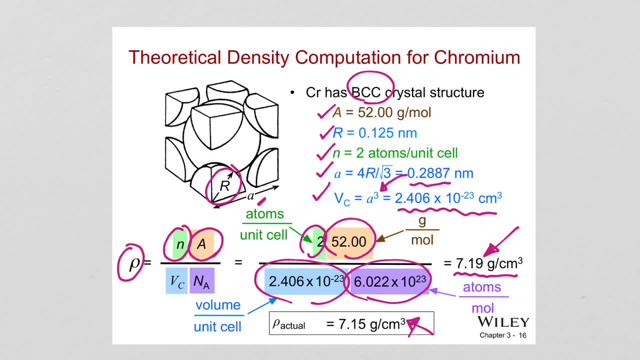 close to what is the actual, what actual number is. so this also tells you if you work on the unit cell level you can very close the approximate, the actual density for you, okay, so if you look at the units also you can understand, because Adams going to cancel, unit, cell gonna cancel, mole gonna cancel and you're gonna end up with 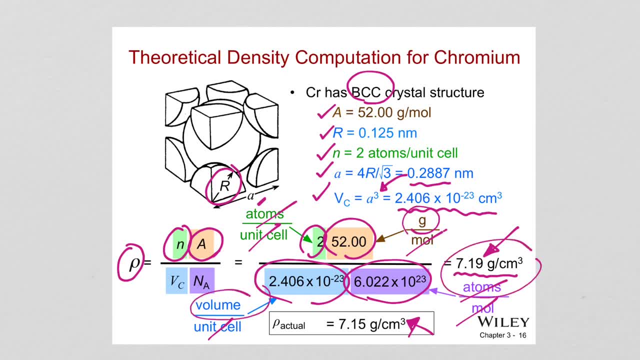 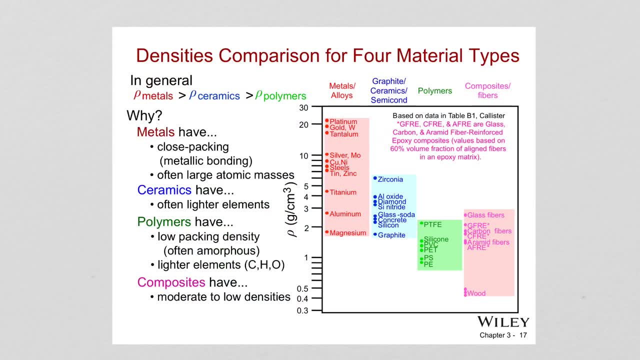 ground per mole. right, this one. okay, in this figure we are given a comparison between metals, allen and copper, ceramics, polymers and composites. In general, the density of metals is the highest, They are the heaviest, Then ceramics, then polymers. Why? Because metals have closed packing like FCC, HCP, And since, think about it, you can fit in more atoms in a unit cell. 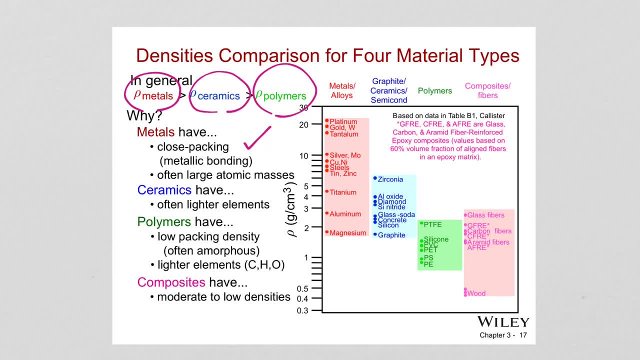 And metals also have large atomic masses, whereas ceramics. often they are light elements, lighter elements. In polymers they are usually amorphous, meaning it is not a very densely packed structure. Remember there is random alignment of atoms in 3D space. if we have an amorphous structure, Therefore there are more empty spaces in between the atoms when it comes to polymer packing. 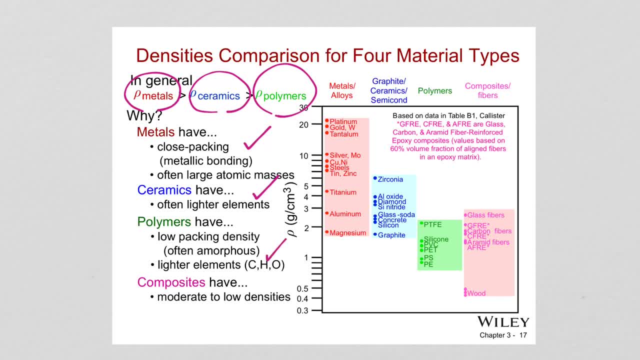 And there are also lighter elements like carbon hydrogen and oxygen, And composites are moderate to low densities because many times the matrix for the composites, the main part of the composite, is polymers, So therefore, if you look at it, it's similar to polymer density. 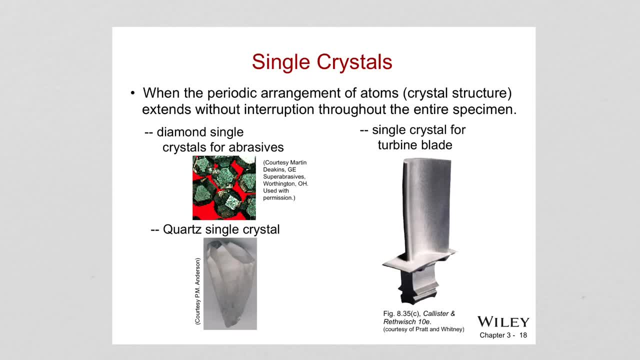 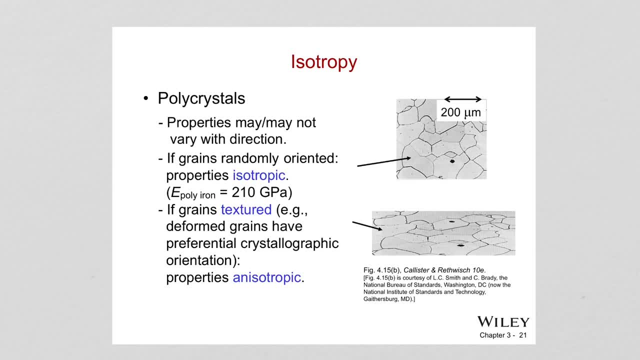 So when the periodic arrangement of atoms extends without interruption throughout the entire specimen- we call it single crystals- may not vary with the direction because the grains are randomly oriented. so we are talking about only a single property here. 210 gigapascal, let's say as an 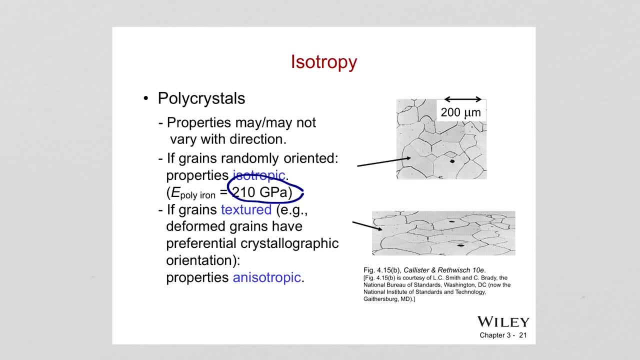 elastic modulus. however, though sometimes so. this is how it looks under microscope. however, sometimes, when we do, let's say, deformation to the overall material, the grains can align in certain direction. if grains can align in certain direction, like, for example, this became like this: right if, if the grain start to 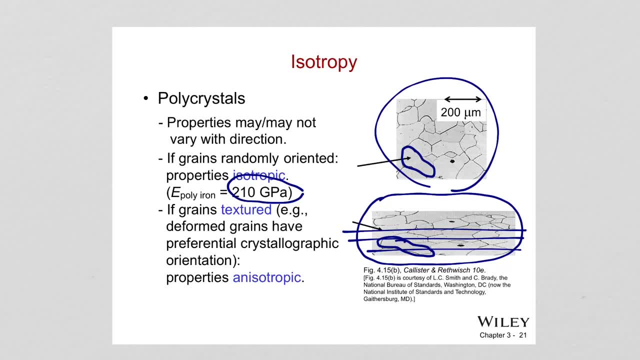 align like this because we did some deformation on it. then still we can talk about the properties changing along one direction- the borders between teleportation andipse. So you can induce anisotropy. if you actually deform the grain structure, The properties may change with the direction. then 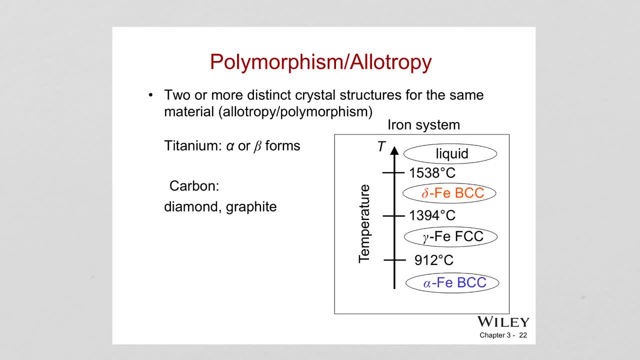 What is polymorphism And it is also called allotropy, That is, if your material can exist depending on the temperature, can exist in different crystal structure, then your material is showing polymorphism. For example, this is for iron. Depending on the temperature, iron can show a BCC structure. 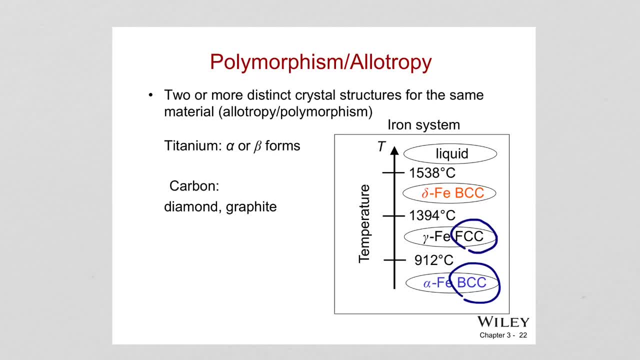 If you increase the temperature it can show FCC And it can go back to BCC As you keep increasing the temperature before it actually melts and forms a liquid And similar to that. diamond and graphite are examples of different crystal structures of carbon. 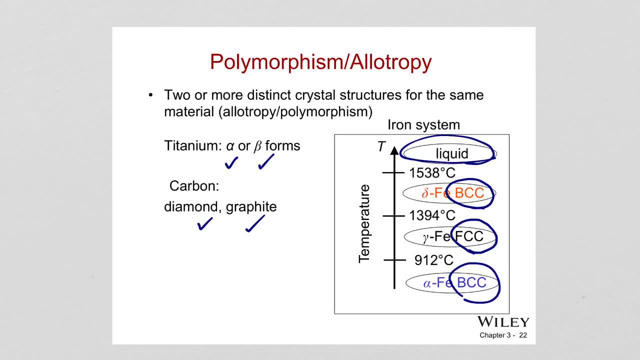 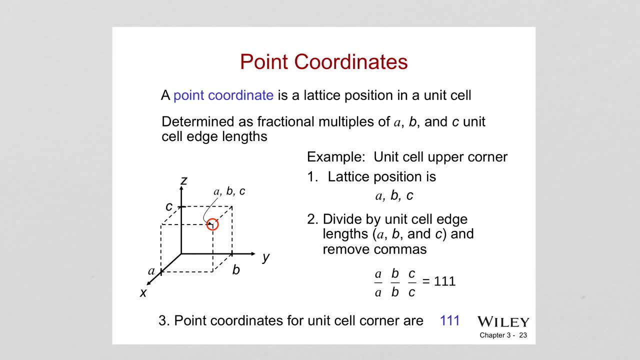 Titanium can also have alpha and beta forms. So when dealing with crystalline materials, it is often necessary to specifically study the material. For example, you can identify a particular point within the unit cell, And this is achieved by crystallographic directions, crystallographic planes. 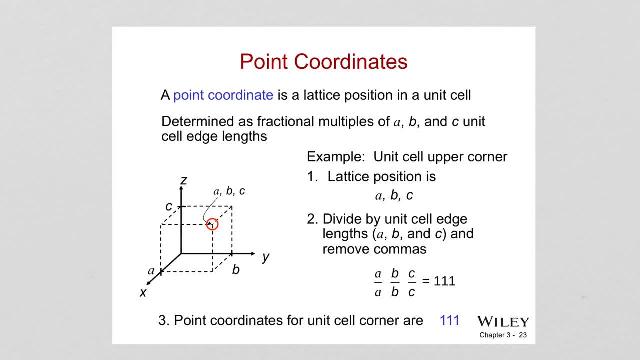 And of course this starts with to be able to define points in space. So let's start with point coordinates. What is point coordinates? It is a lattice position in a unit cell. So three: d, x, y, z Axises. 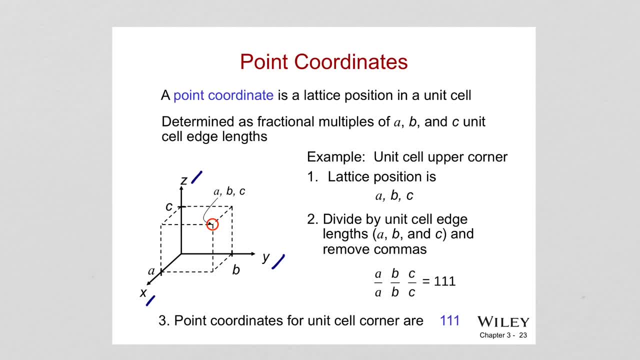 Vertical. here is our unit cell shown. okay, so it is defined by, basically, fracture multiples of a, b, c unit cell edge lengths. so this coordinate is a right. this coordinate is b and this coordinate is c. so therefore, if we try to write a point coordinate for this, it's going to be a, b, c. but how we need. 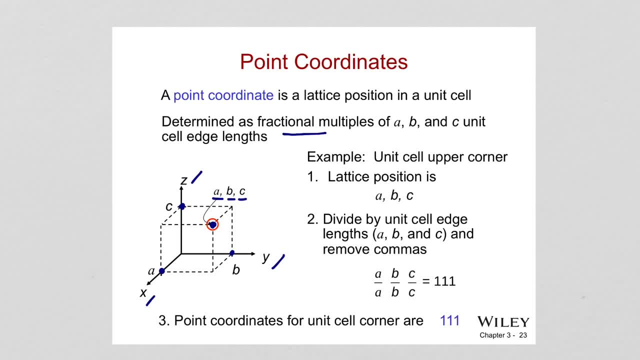 to define this is: we need to define this to the length. so this length is a, this length is b, this length is c. so therefore, first identify lattice position and divide them to unit cell edge lengths: a over a, b over b, c or c, one, one one. so the point coordinate for this point is one one. 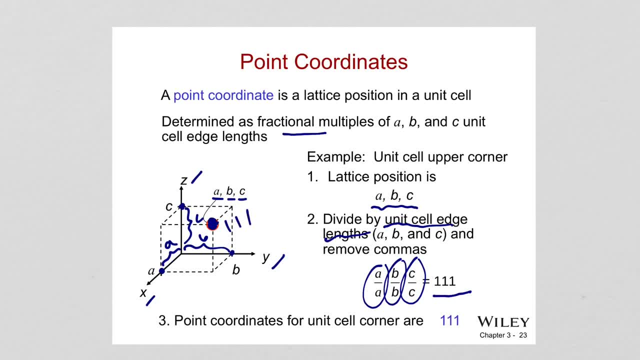 one. I usually think about this as that. So to reach the point 1,, 1, 1.. So let's erase this. So how much I need to move along A, B, C axes, A B, C directions to reach this point? This point is where I'm trying to reach. 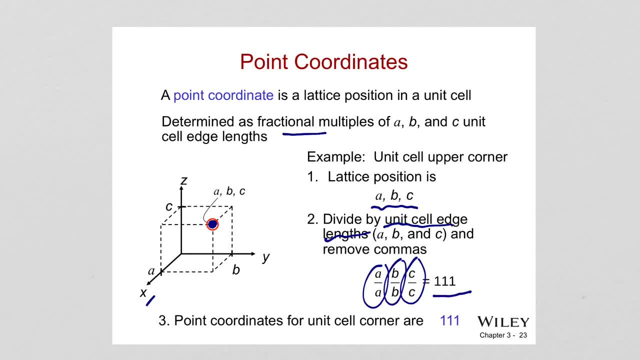 So I need to move 1 times of A to reach here first and 1 times of B to reach here and 1 times of C to reach here. So that means 1,, 1, 1.. That is a way to go. So this is for just understanding what is each point coordinate in a unit cell. 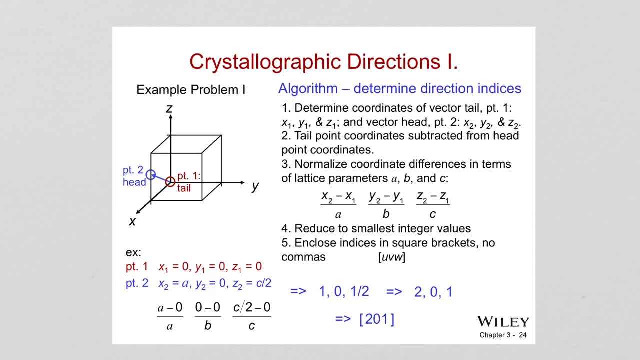 So when we are defining crystallography directions first in the unit cell, the direction will be drawn to you and what you need to know is the one first. let's say: this is our direction. right? we need to know first the point coordinates of the tail and point coordinates of the 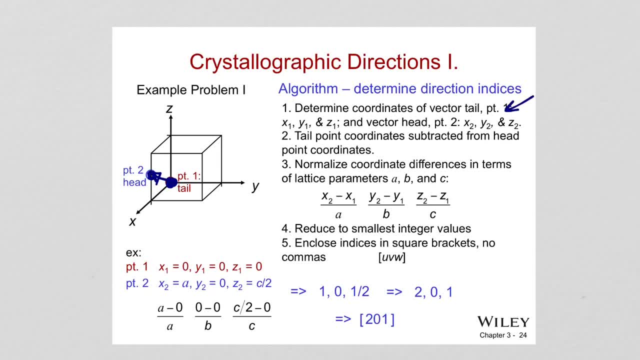 head. that's what you do first, okay, step by step. and then subtract tail point coordinates from the head coordinates. so we have for tail 0 0, 0, because we are at the origin right in this place. this is the origin for point to the end head. 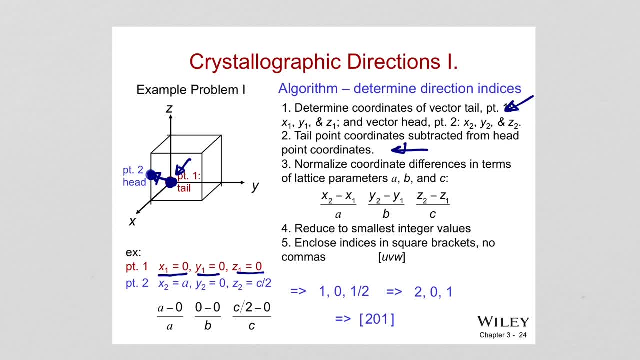 what is the coordinates? so it is. I need to move one times one, so it is a. or you can say the point coordinates are one. I moved one times, ok, one, and then I don't move along the y-direction, so it is 0 and i need to move in the LZ direction one over two. 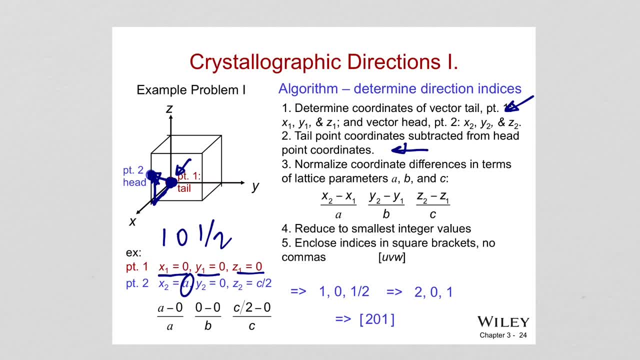 ok, but i need to get rid of fraction so i need to multiply each term with to 201. if you multiply each of these with two is going to you to 0, 1, so to 0, 1. ok. so the point coordinates of the origin, the tail, 0 0, 0, and the point coordinates of the two head is 2 0, 1. so 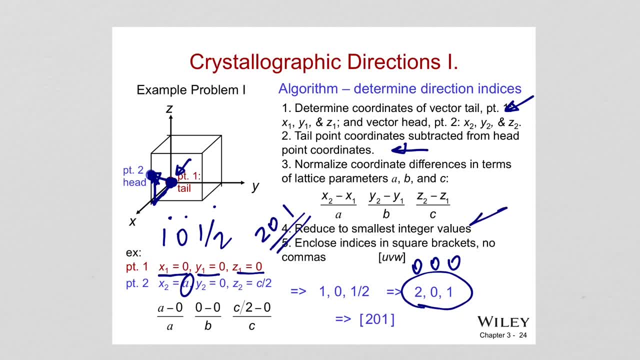 don't forget to get rid of the integers. okay, and then now what we need to do is subtract. subtract tail from head. okay, so 2 minus 0, 2 0 minus 0 0, 1 minus 0 0, and then we show it in square brackets like this: this means 2. I'm sorry, there is a mistake here. 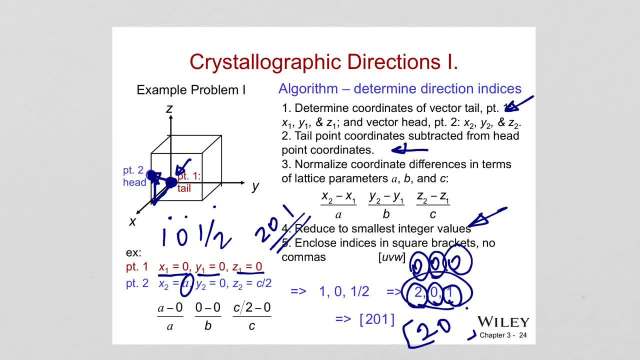 so 1 minus 0 is 1, so it is 2 0: 1 direction, and we show it with like this a in square brackets. so what we find is actually this one: this direction is 2 0: 1 direction, and we show: 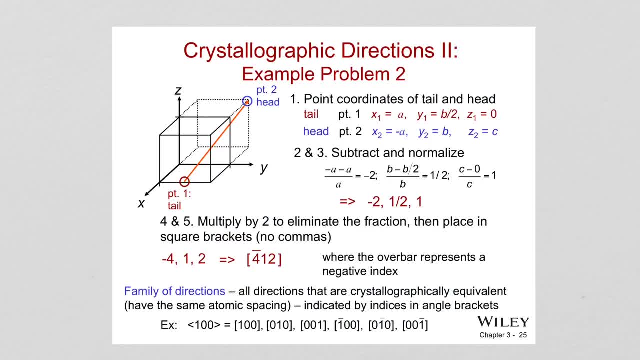 it like that. another example: let's do it together. okay, let's look at the head, head and tail point coordinates. to reach the head point from the origin, I need to move minus 1 along the X, 1 along the Y and 1 along the Z. so that's the point coordinates of head. 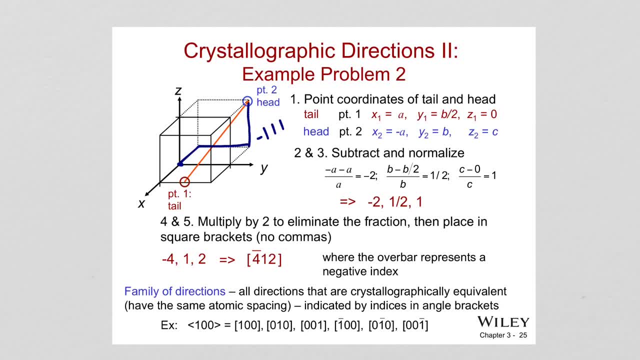 what about tail? it is I need to move from the origin: 1 on the X direction, 1 over 2 in the Y direction and 0 in the Z dimension. so need let's subtract them from each other. minus 1 minus 1, minus 2. minus 1 minus 1 over 2, 1 over 2 and 1 minus 0 is 1. okay. 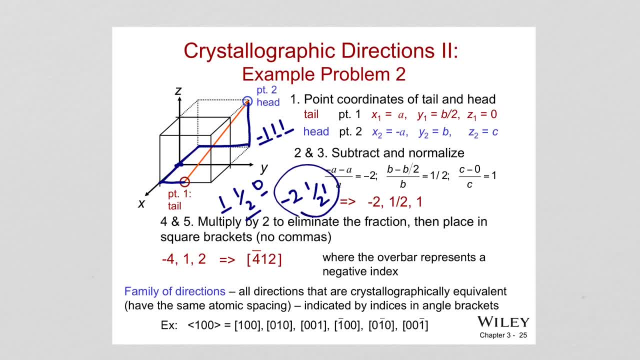 so we need to multiply this with to get rid of the fraction with 2 right. so it will make 2 times minus 2, 4.. And 1 over 2 times 2, 1. And 1 times 2, 2.. So here is your. 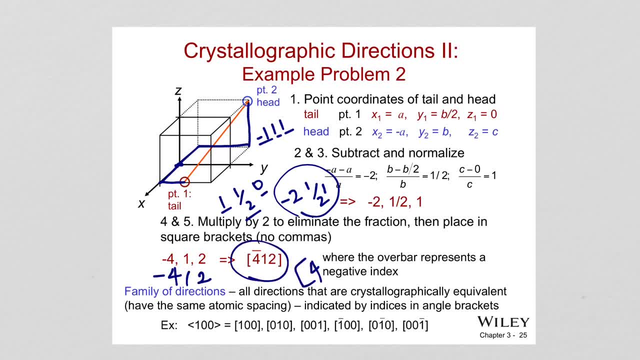 direction We have 4.. So negative to show negative, we have present as an over bar like this: 4, 1, 2.. So there are family of directions that are crystallographically equivalent directions that has the same atomic spacing. So it means depending on 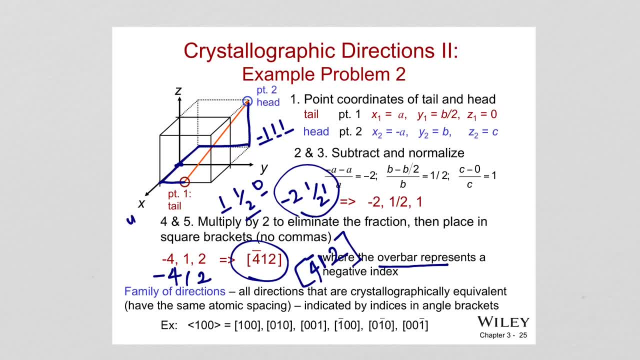 how you choose X, Y, Z. Someone can say here Y. Someone can say here Z. right, Depending on that, how you define the direction will change And this will tell you that these are crystallographically equivalent directions, For example, for 1, 1, 1, 0, 0. 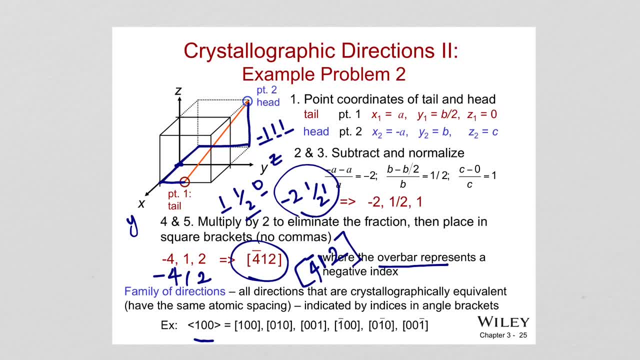 family. So if it's family, it's gonna be angle brackets like this. so one zero zero. family represents the directions. one zero, zero. so let's say zero one, zero, right zero zero one or the negative ones: one minus zero, zero, zero, one minus. 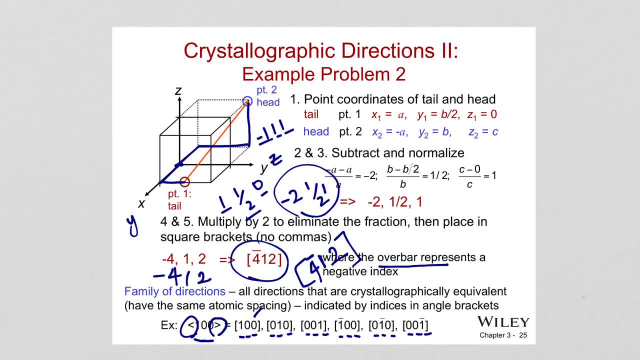 zero, zero, zero one minus. so all of these, depending on how you define x, y, z, the place of the one changes and also the equivalent ones. are there negatives? they also equal and they crystallographically equal. so I suggest you, guys, if you are having hard time imagining these directions and these, 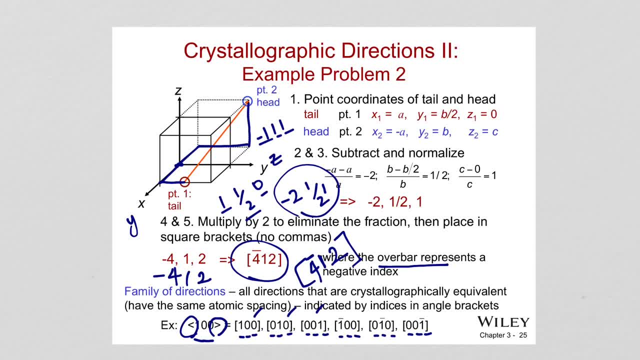 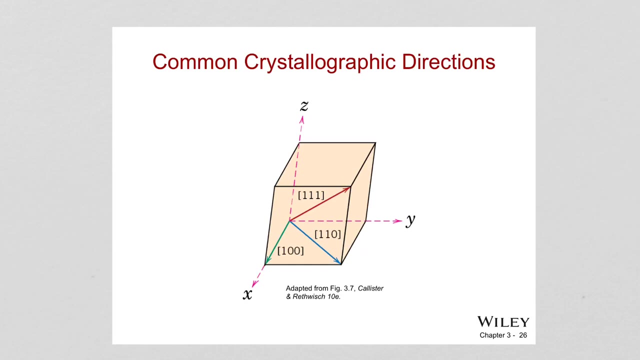 families. you can google the saying one zero, zero, family of directions and you will see that there are images where these directions are drawn on the unit cells and this can. you can visualize it, okay. so common crystallographic directions, it's one zero, zero, one, one, zero, one, one one, and we have just seen how to write one one one. 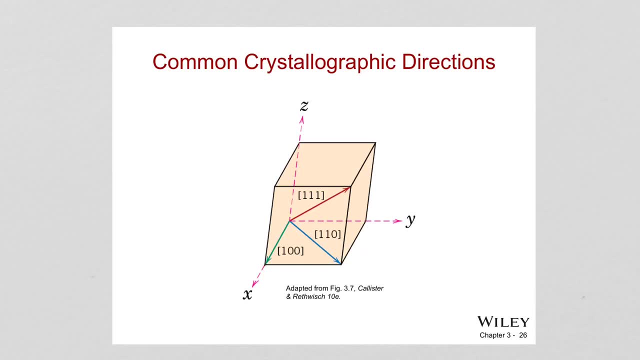 and one one, zero. if you guys want, i can just do it now. for example this: this point is one, one one and this is zero, zero, zero. and one minus one, one minus zero, one, one minus zero, one, one minus zero one. so this is one one, one direction. this point is one one, zero. uh, point coordinates. 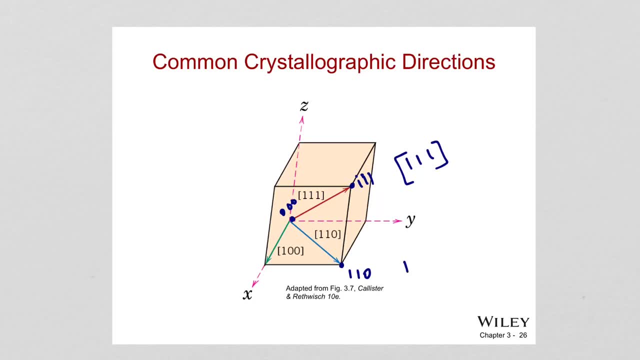 this is zero zero, so one minus zero one, one minus zero one and zero minus zero zero. and then this point is one zero zero, and then this point is one zero zero, and then this point is one zero zero and one minus zero. one zero minus zero, zero, zero minus zero zero. and this is the one zero zero. 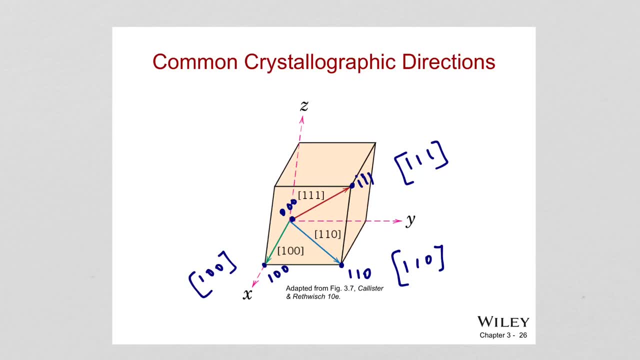 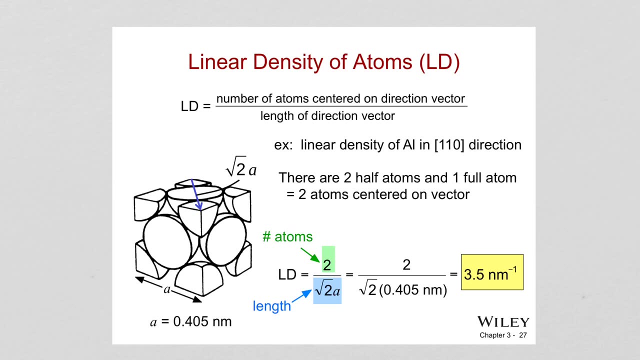 direction. okay, so linear density of atoms. so if we want to calculate a linear density, let's say for an aluminum atom in a certain direction, let's say one one zero direction, and then first we locate that direction in the unit cell. it's gonna be one one zero direction, right there. 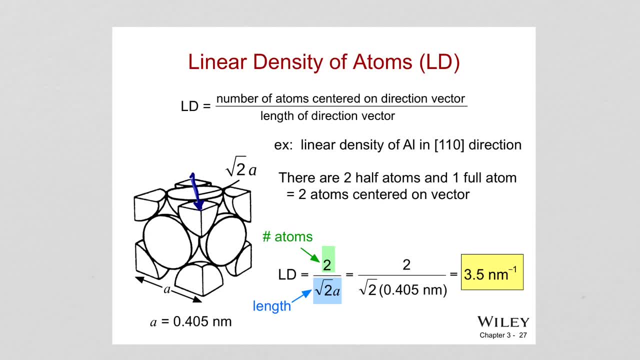 and then we need to calculate, let's say, linear density and how it is defined, basically along that direction it tells you how well the atoms are packed right. so if you look at that, you will see how many a number of atoms centered on the unit cell and how many atoms are centered on the unit cell. 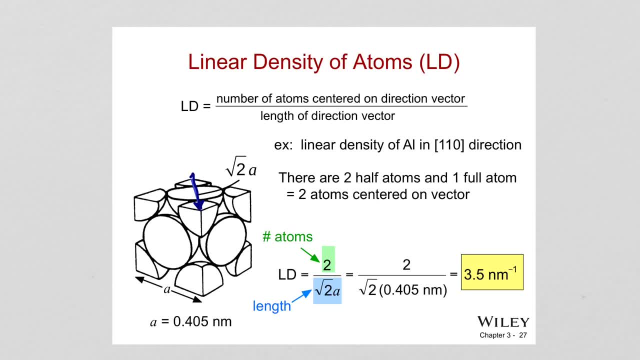 on on a direction vector and length of the direction vector over the length of the direction vector. so to figure out how many atoms i would suggest, if you guys look at the atomic radius right. so this first one is r and this in the middle two r and this one is r. so that means 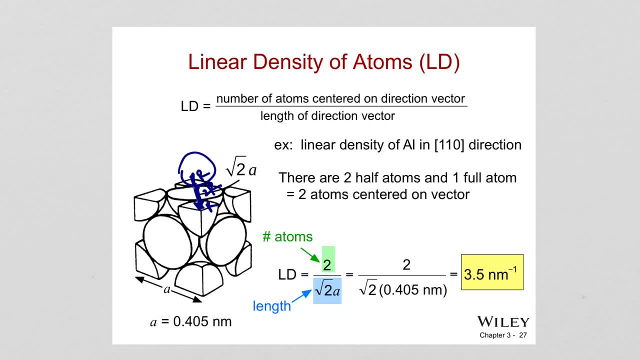 these are half of the one atom overall here represented. this is one half of the one atom overall because the diameter is two r right. so r and r makes one atom. so there is one full atom and then there is this one r. this is one full atom at the center two r and two half atoms. 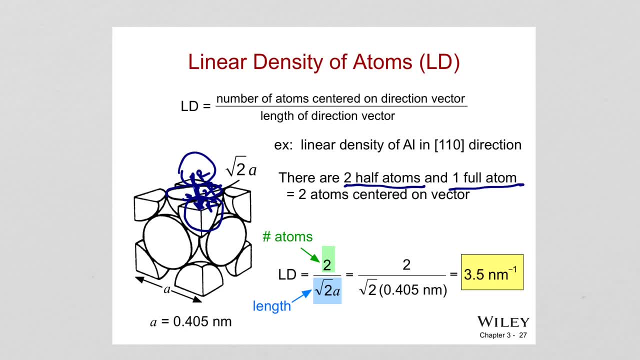 makes uh, one full atom, so there is two full atoms centered on the vector. so you put that number here and of course divide that to the, to the length, and the length is, of course you calculate: this is a, this is a, this edge, is this this length of this? 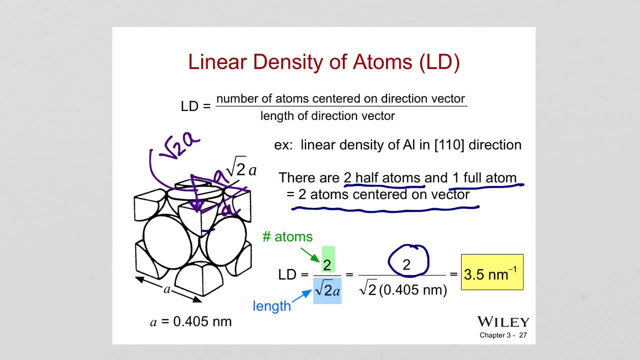 vector is two square root of two times a. so plug in that in, and a is, of course comes from the unit cell dimension of aluminum. it is given, right, it is given. so you just calculate it and you find that. you find that you will be able to represent the what is the linear density of atoms. 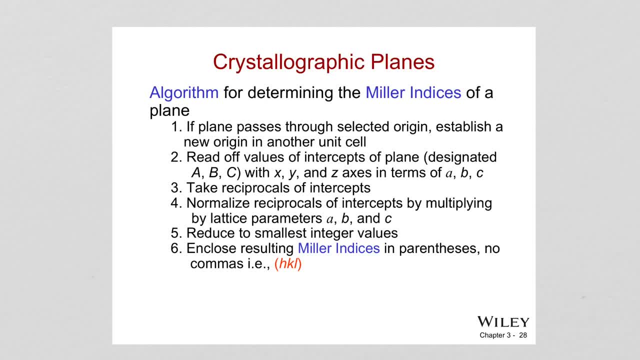 so, when it comes to crystallographic planes, how we will represent crystallographic planes. so there is, the strategy is summarized and then i'm going to show it. first, you need to figure out where your origin is and in the unit cell, and if the plane is. 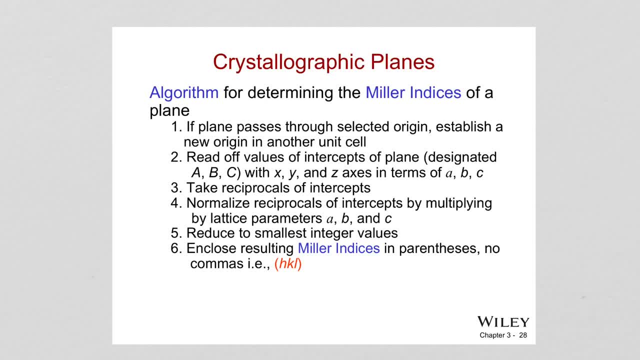 origin and then you need to choose another origin, okay, and then you need to read the values of intercepts of that plane in XYZ accesses in terms of ABC, and then take the reciprocals and then normalize it, get rid of the integers, and then you will be able to write them. represent the crystallographic planes. 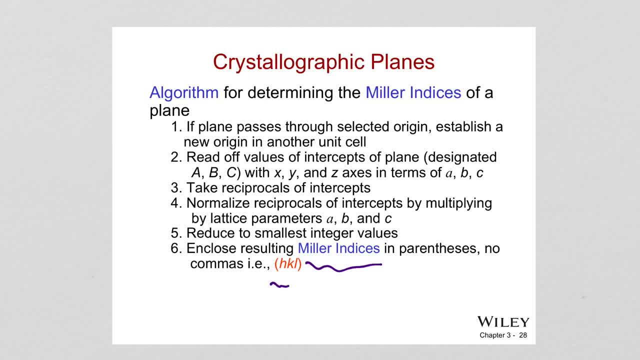 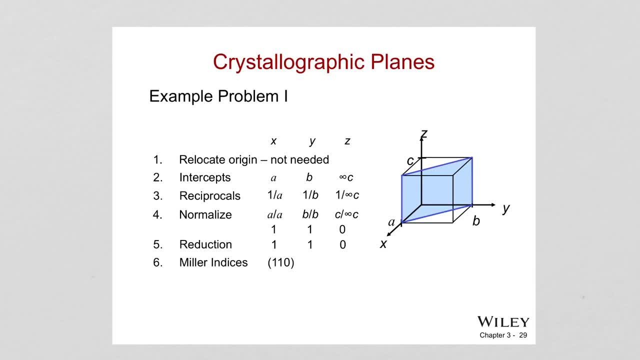 what we thought we called Miller indices HK. yeah, okay, let's do it so, okay. so how do we define crystallographic things? there is the example here, so I would follow this procedure that I'm writing down here. so, so write XYZ, okay, so first check if the origin, if the plane is going through the origin. no, so it. 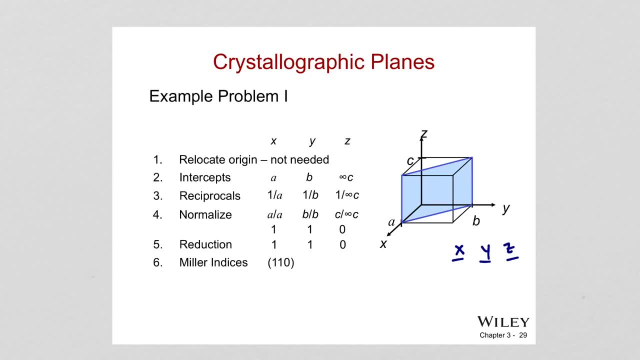 doesn't have to be relocated. so where does it intersect XYZ? okay, so it is intersecting X at a that is 1 times of a right. so I write one, and it is intercepted at 1, 1, and it is not intercepting Z dimension at all. so we write infinity, okay. so now what I? 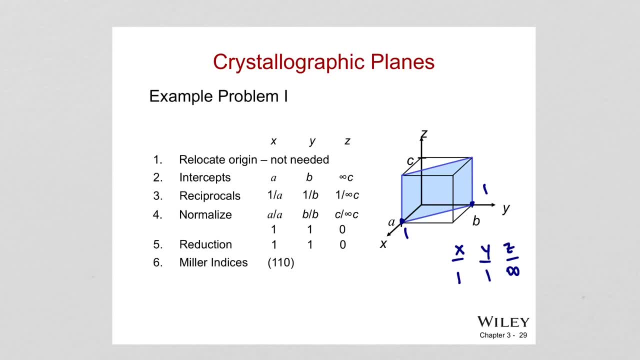 would do is: I would take the reciprocal of this to get rid of that infinity. so 1 over 1 1, 1 over 1, 1, 1 over infinity is 0, okay, so is there any fraction? no, therefore, you're gonna read the Miller indices: 1, 1, 0 plane. so this represents: 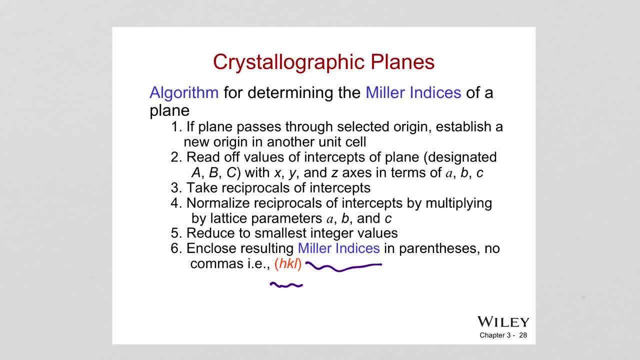 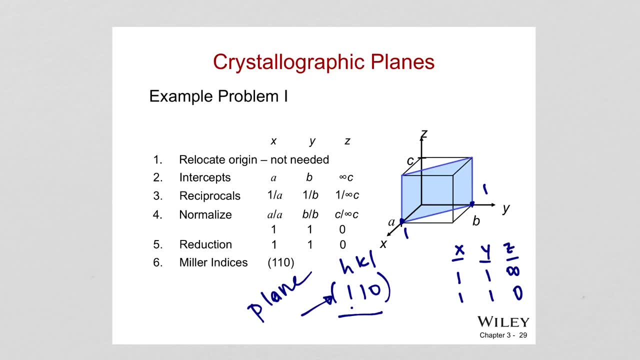 plane, so parenthesis plane. it's also called HKL plane or 1 1 0 plane. so HKL is like representing the Miller in this indices, in this case Miller indices 1 1 0. so this is how I would do it. so another one here. let's do it. 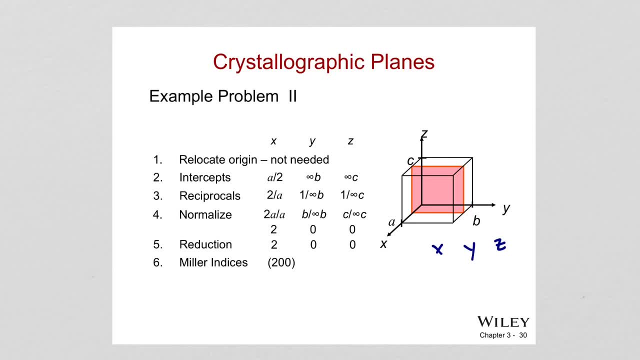 where does it intercept a 1 over 2? where does it intercept Y infinity? where does it intercept Z infinity? take reciprocals 2 0, 0 so you find the Miller indices 2 0 0. that's a 2 0, 0 plane. okay, another problem here. 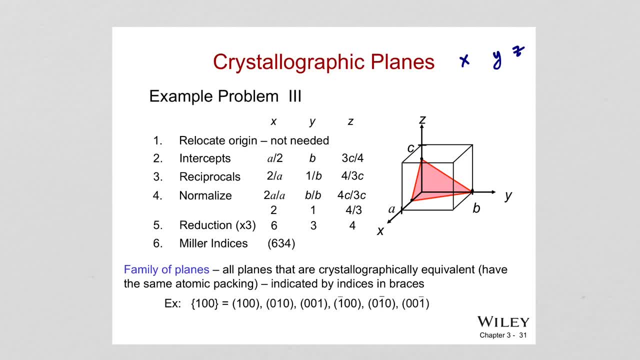 let's look at it. where is the plane intercepting a approximately? it is not exactly given, but I'm guessing it's 1 over 2. why is 1? Z is, it seems, like 3 over 4? but it should be more clearly defined here like that. okay, so take the. 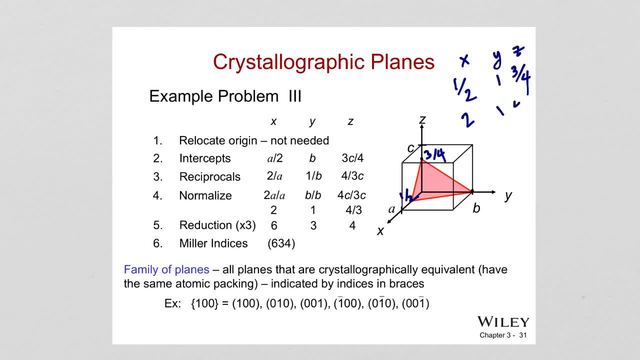 reciprocals: 2, 1, 4 over 3. we need to get rid of the fraction, so we need to multiply, multiply, multiply, multiply each with the three, this is gonna be six, three, four. so your plane is six, three, four plane. of course, some planes are crystallographically equivalent planes. 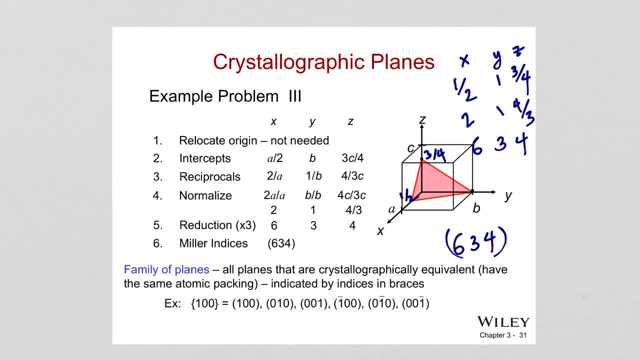 they have the same atomic packing and similar to direction. you can also write it down. so if you see this parenthesis here, this one, it will represent plane family. so one, one, zero plane family represent one, zero, zero, zero, one, zero, zero, zero, one, depending on where its XYZ axis is, and of course they are. 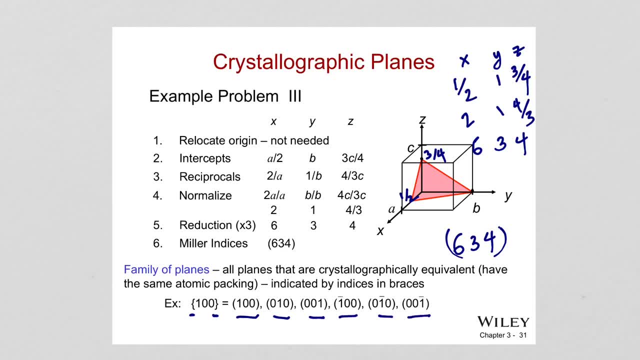 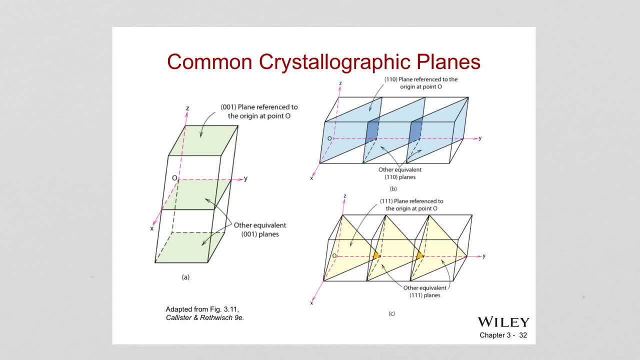 negatives. and here they are, given some visualization so you can understand actually what family means: write you saw they family is. so this plane here, depending on the system, is zero, zero, one plane, depending on how you move the xyz. this plane and this plane and this plane is actually the same thing, right, crystallographically equivalent, or this plane, this plane, this plane. 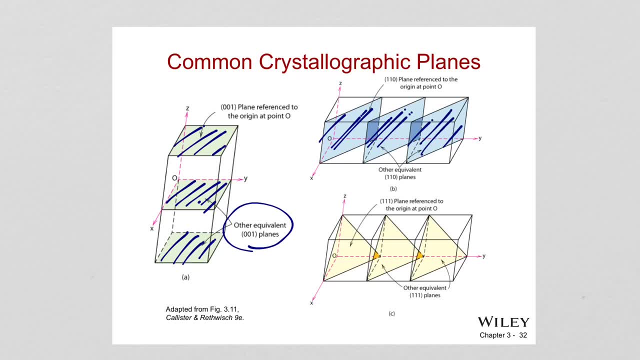 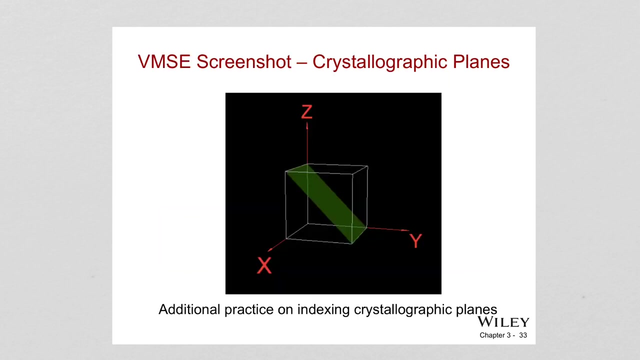 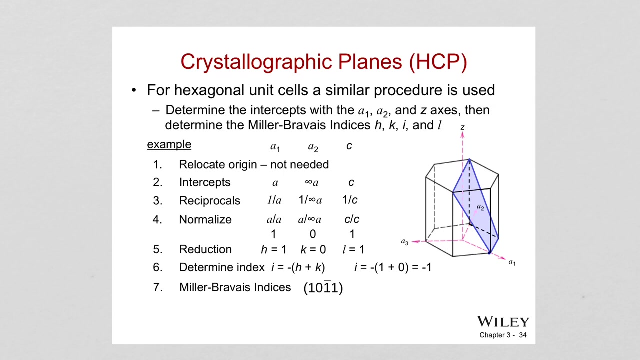 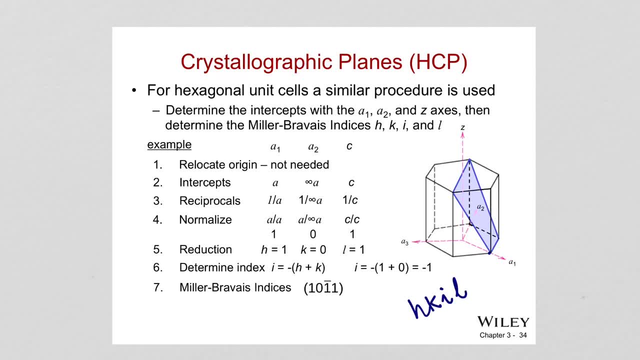 formulae, similar indices and there is a relation here. the i is actually minus h plus k. it is done similarly to the previous examples. here you need to look at where the plane intersects the xyz. okay, so i would write a1, a2 and then a2 and then. 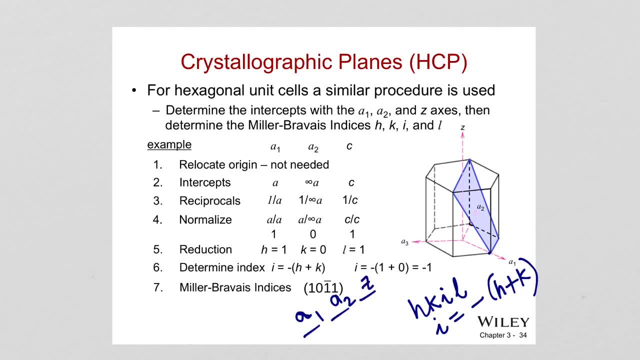 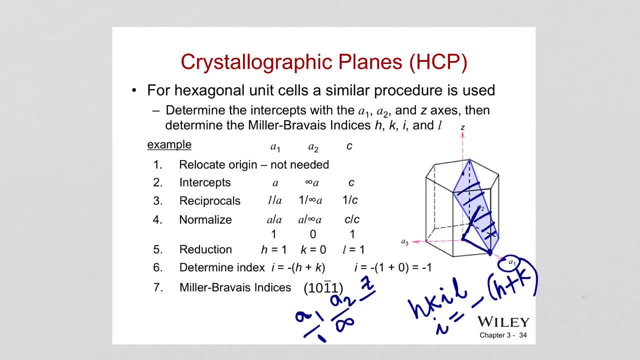 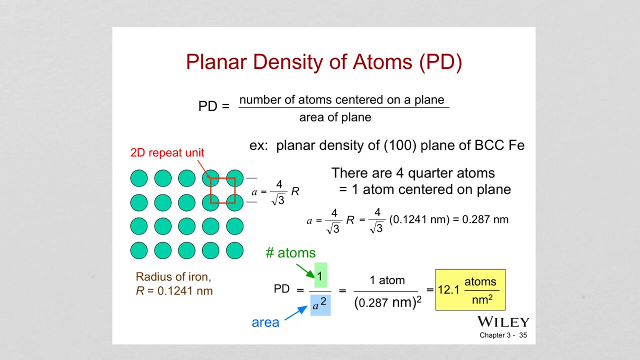 with a2 at all. so infinity, what about this? it is intersecting at one times of c, meaning one. of course we need to get, so if we don't have enough of the, the, and if we need, if we need, so, if we need to calculate planar density of atoms. 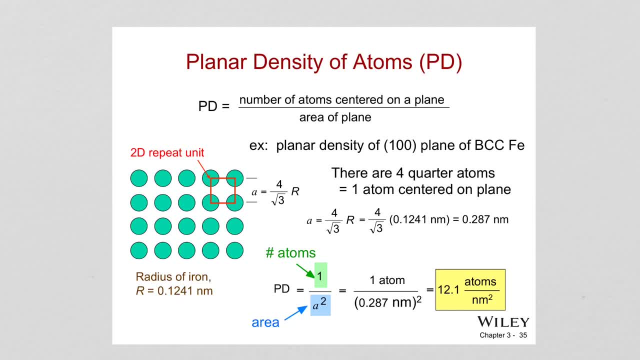 that means in one plane how many atoms are fitted basically. So it is done by an equation: number of atoms centered on a plane, over the area of plane. So let's say we are trying to figure out planar density of 1,, 0,, 0 plane on BCC ion. 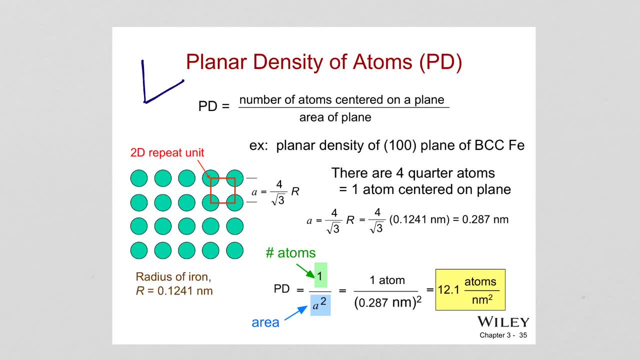 So if you look at the- I'm sorry- unit cell of BCC 1, 0, 0 plane, is this one right? and we know atoms are at the corner in this one and there is one at the center, but there is this one at the corners. this one is this actually. 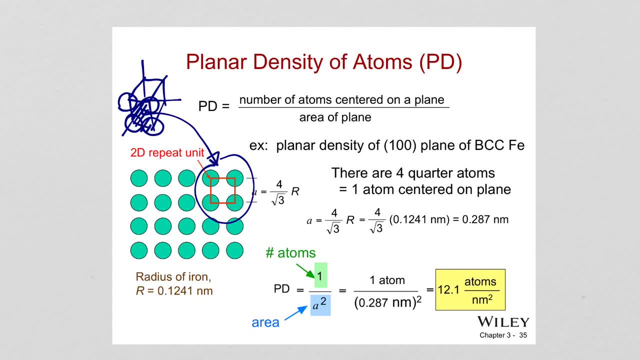 and we are looking at 2D and 1, 0, 0 plane. we are looking at and we are seeing actually 4, 2D quarter atoms. that means there is one atom centered on the plane, just one atom, and then we know the number of atoms, then 1. 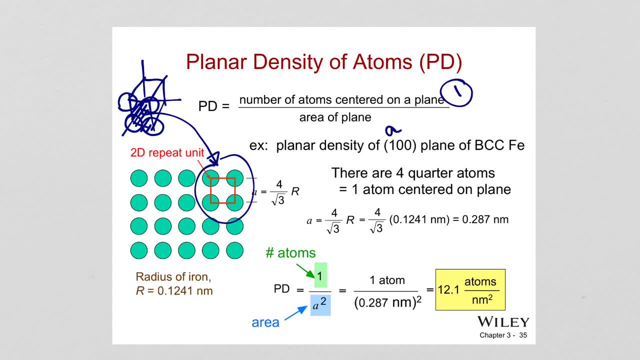 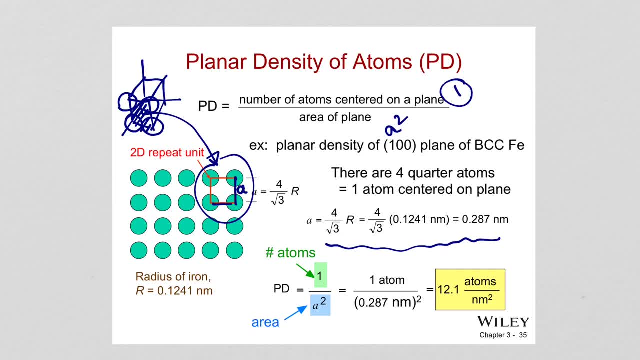 if we look at, this is A right, this is A, and there's the body diagonal. this one, you guys remember we found this relationship for BCC between A and R. this was body diagonal, right from the body diagonal, which was this we were able to find. it was for R and from. 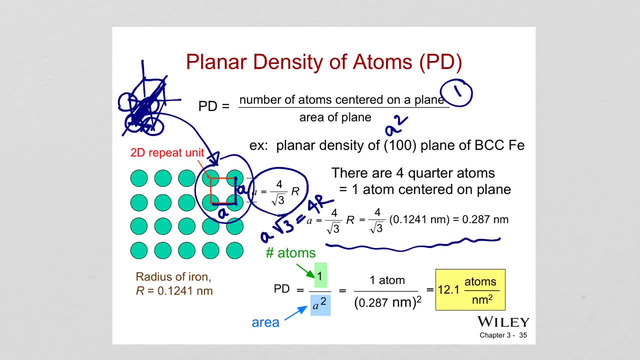 that there was this relationship between R and A and since we know A, you can calculate, since we know R, you can calculate A. so once you found A, the R is given. this is the radius of iron atom. you can put it in and put it in here and 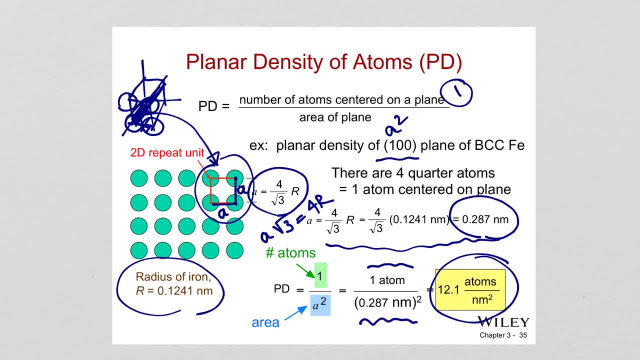 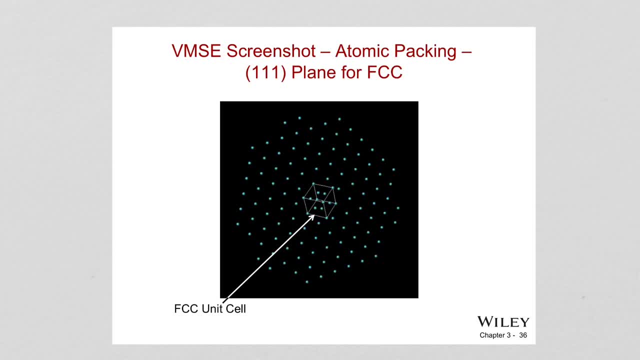 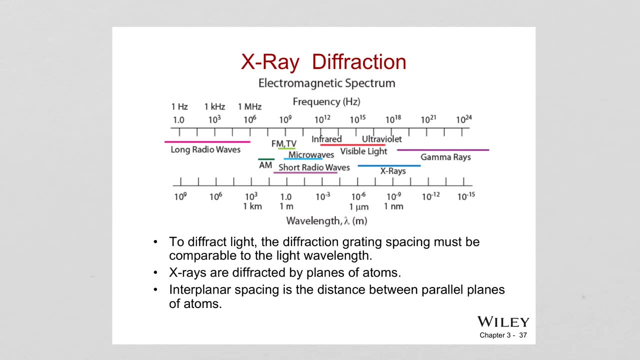 calculate the planar density in 1, 0, 0 plane of FCC. X-ray diffraction is very important technique that gives us information about the crystal structure of the material. Like you can figure out if the material is VCC, FCC, how the atom is packed. 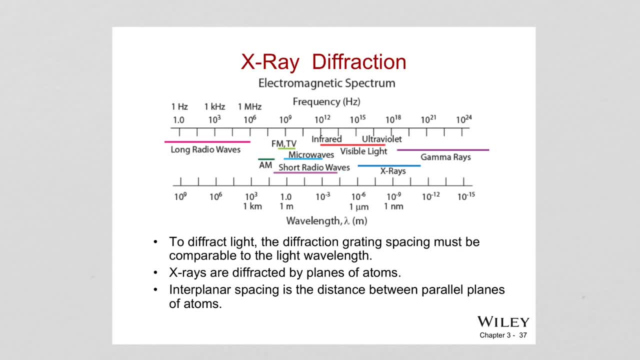 So a lot of the information we know about materials comes from X-ray diffraction. The reason is that if you see the X-rays here in electromagnetic spectrum, the wavelength, it is because the wavelength of X-rays is comparable to the interplanar spacing. 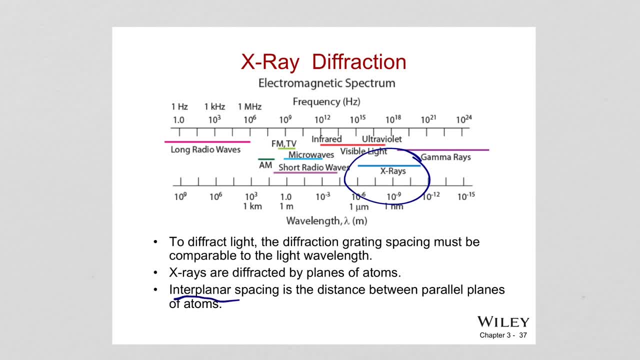 So space in between, space in between the X-rays and the interplanar spacing Planes of atoms, And therefore what happens here is X-rays are diffracted by the planes of atoms And this way, when we sense that diffracted X-ray, we can obtain information about the crystal structure of the material. 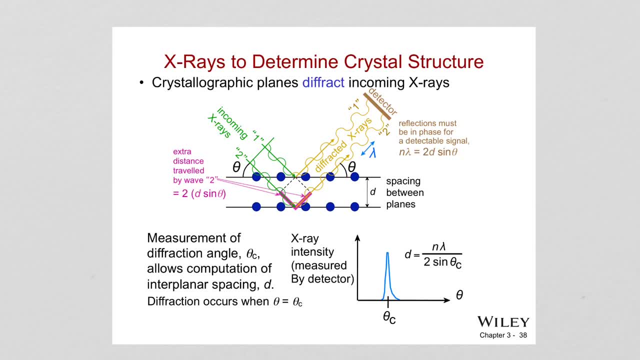 So here is how X-rays are used to determine crystal structure and how they diffract. X-rays are diffracted from the crystallographic planes, So you see two crystallographic planes And then there are atoms. These are atoms And the spacing between the planes is D. 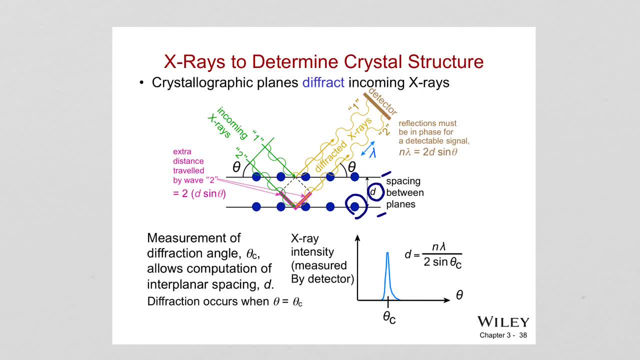 Okay. So what happens here is those X-rays: when diffracted see- with the green we are seeing the incoming rays and the yellow ones are the diffracted. X-rays are diffracted from the crystallographic planes. And when X-rays are diffracted, they need to be. they need to be interfere constructively And because otherwise, if they don't interact, interfere constructively, then they will cancel each other And at the end, when it comes to the detector, you cannot see anything. 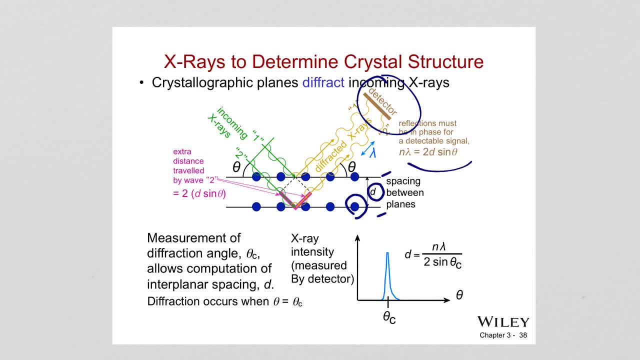 So therefore, this is a very important point. So therefore, this condition has to be satisfied. That means that means that when they travel they need to be in phase, meaning they need to interfere constructively. So the total distance traveled that has to differ by a whole number. multiple of their wavelength means. so if you look at the first ray and the second ray, 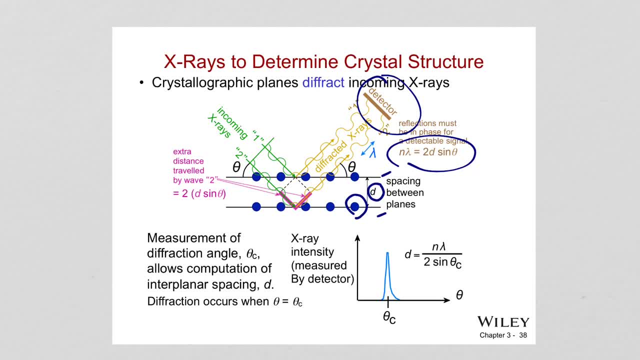 you're going to see that there is an this part and this part is in phase, meaning they interfere, interfere constructively, but there is an extra distance traveled with the second incoming ray incoming ray. So what is the distance This distance traveled has to be? 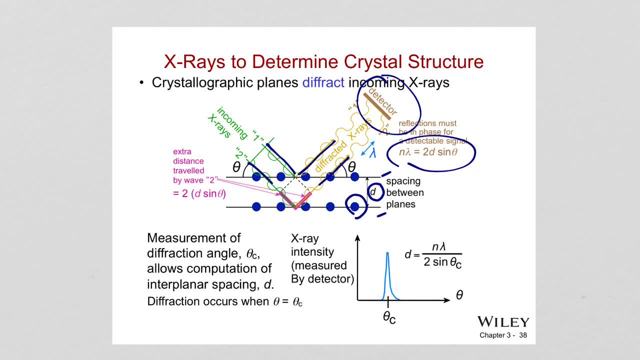 a whole number, multiple of the Burke length. So this is the reason you can have in: the detector Can detect these X-rays, otherwise they will cancel each other. So a whole number of wavelength. So if this is the wavelength From here to here, right, 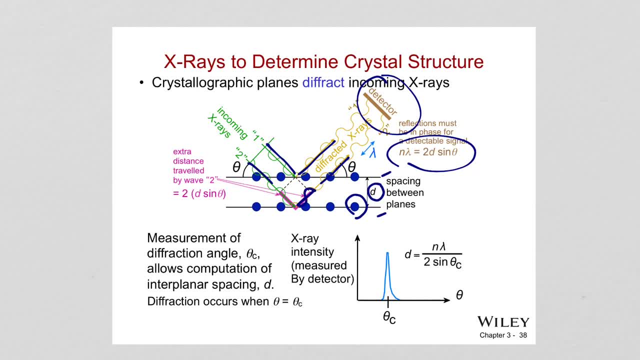 This is the rate, So it has to be this extra distance traveled here has to be the integer multiple, has to be the integer multiplication, has to be the integer multiplication n of the wavelength, otherwise they will experience a phase shift and these two 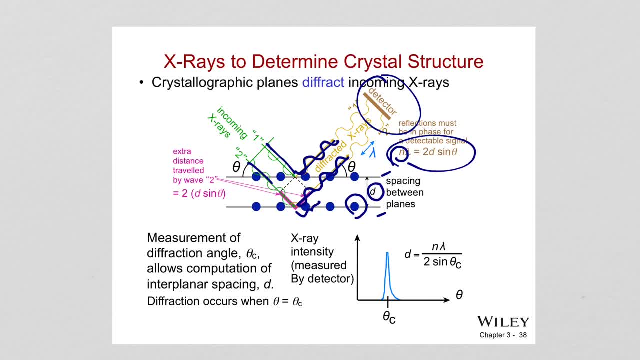 rays cannot interfere constructively and then we cannot see it. so these conditions we called Bragg's law. this has to be satisfied. so this extra distance travel, so let's figure out what is the extra distance travel has to be, again, mal integer multiple of the wavelength. so this is D right and this 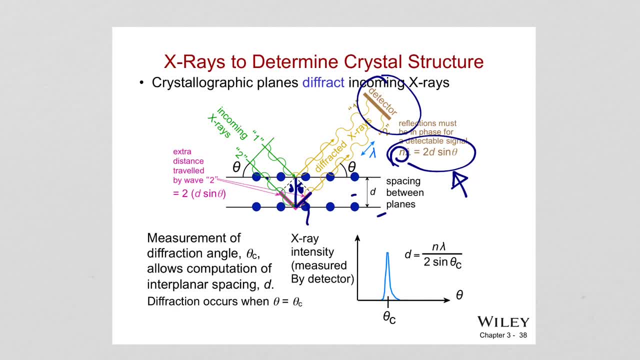 is theta and this is D times sine theta. but we have two of these extra travel distance. so two times D sine theta has to be integer multiple of the wavelength, otherwise these rays cannot interfere constructively, cannot add to each other. they would cancel each other if this condition is not satisfied. so this is called Bragg's law. so when? 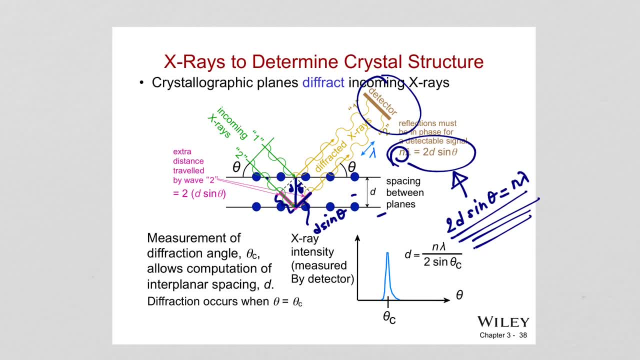 this happens at a certain angle, these diffracted beams, they interfere constructively, meaning this one is like this, another one is like this, the same phase, so they add up and then what you detect in the detector is a peak like this. okay, it's a peak that is happening at a certain angle, when the x-ray is basically 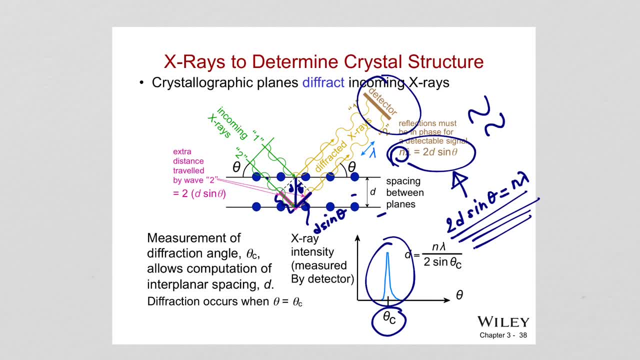 incoming at a certain angle. they can adjust a different angle, send the x-ray beams and at that angle they record a peak and that means at that angle there is constructive interference. the way we can add up the diffracted beams and that we satisfied dengan ilikas Anthony Bergemann. 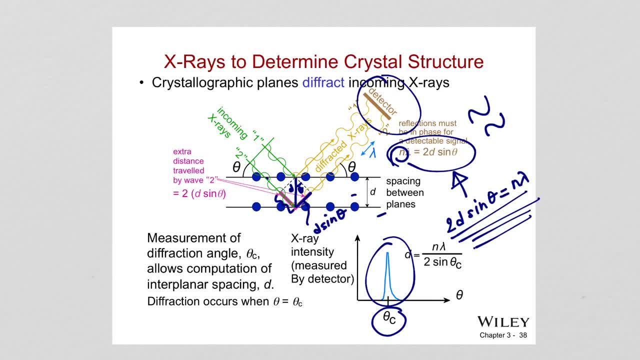 Since Bragg saw with us this information about a 헤izik dumbbell, batter mas cameras, and that we satisfied the Sleep & Gain program by connecting this with us and by find the Bragg's law and that angle. now, using this equation, we can figure out: 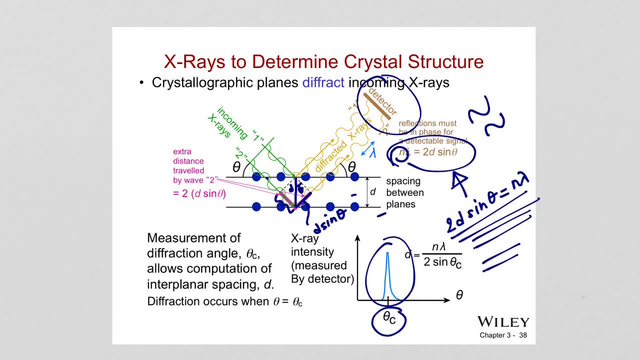 what D is, because n is is gonna be always integer and the lambda is known from the x-ray device. okay, and then the angle we calculate from the detector D we find. so it is too much detail, but it doesn't matter. what will you? you give it. 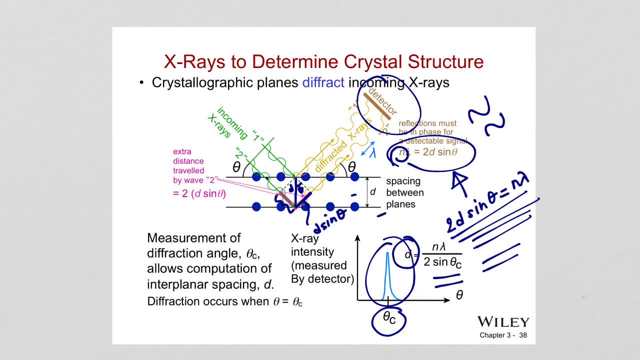 to n. okay, n is equal to 1 is acceptable because at the end it is always gonna be compensated in the equation. let me tell you that way so you can accept n as 1. okay, and don't forget to subscribe to my channel and turn on the notification bell so you don't miss my next video. Thank you. 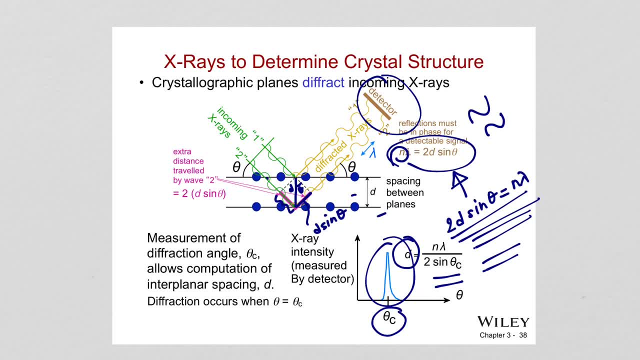 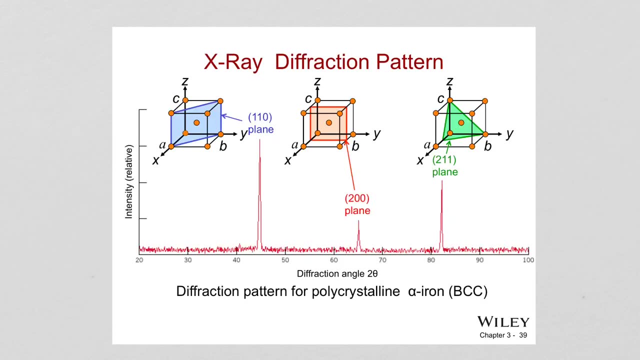 worry about the end. so through this Bragg's law you can easily able to calculate what D is interspacing between the planes by just doing x-ray diffraction. so here you can see that how different planes in a BCC crystal show up as peaks. 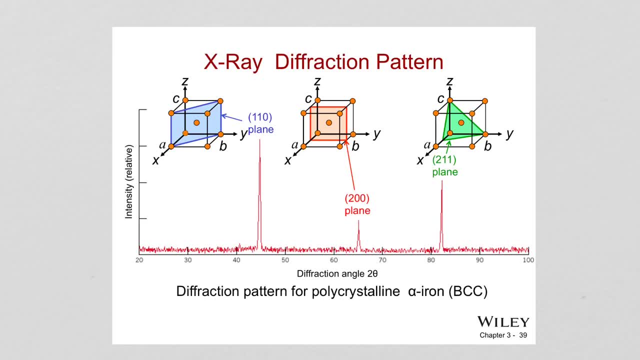 in the diffraction spectrum. so this is a typical diffraction pattern. that result is result of an experiment when they are trying to figure out what the crystal structure is for a certain metal. so from 1: 1, 0 plane there will be a diffraction. from 2: 0, 0 plane to 1: 1 plane, there will be constructive. 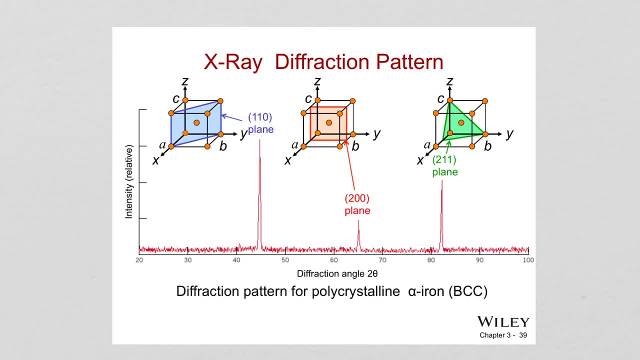 interference patterns and this is how we are seeing it in the x-ray. so from the angle that we observe the peak, we are able to calculate the spacing, and the spacing will actually give you idea about the HKL, meaning the Miller indices. okay, and this equation is actually given as like: 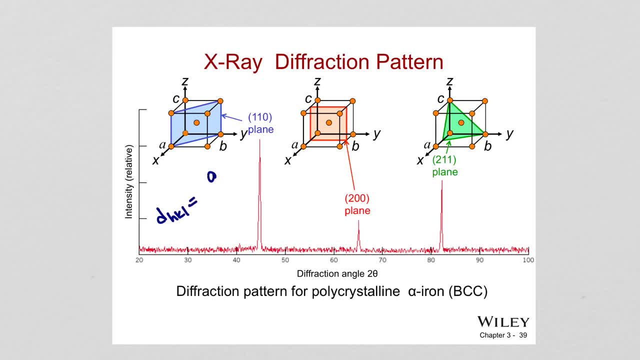 that P and you can also find out peak jaw is slight. so in this equation, like as I said after this, we are surely will be protection in the group screws. that is based on the け, and here you can see that the peak value is a lot, while the amorphous 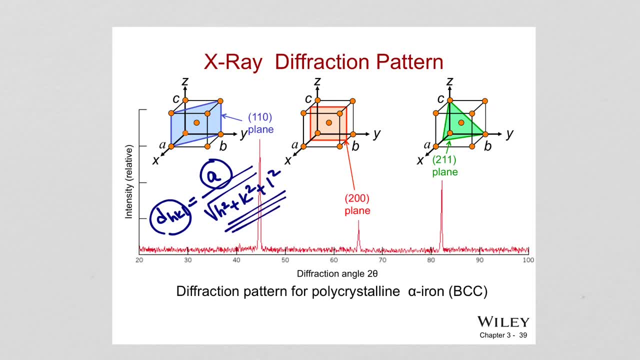 ibile of that extremely nonveg 아니에요 here. so once you know what the D is from the Bragg's law, you know the a plane. so during the week i will send you guys- uh, certain, i will solve certain problems- and then you guys can understand more, if there is a problem, how you can approach the problem. 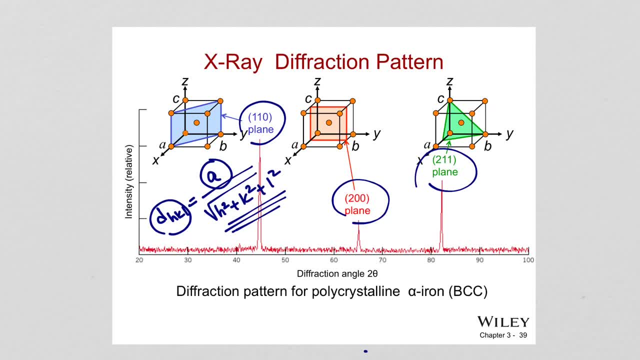 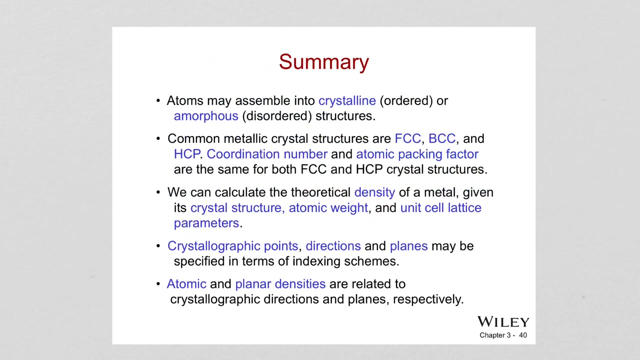 and solving that problem, x-ray diffraction problem, and also i will do some examples on the uh crystallographic directions and planes and directions and point coordinates. um, okay, guys, i think that's it. and then the summary is basically we learned 3d arrangement of atoms in space. we said: crystalline, can there, can be crystalline. 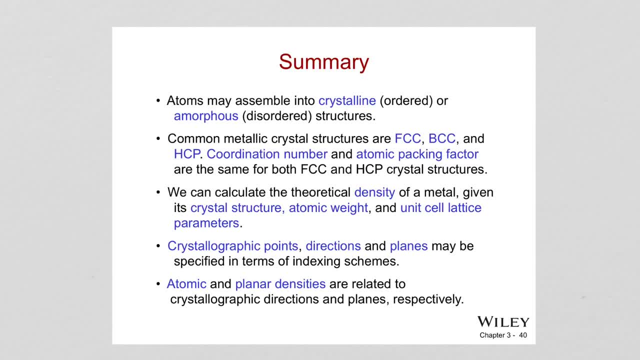 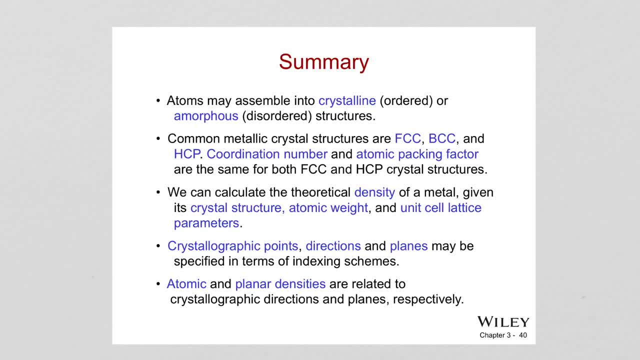 bcc hcp. we looked at coordination number, atomic packing factor and we found those are same for fcc hcp. we calculated the theoretical density and, using information such as the crystal structure, atomic weight unit, lattice parameters, we learned about how we define certain points, direction planes in a unit cell and we also learn atomic and planar densities.